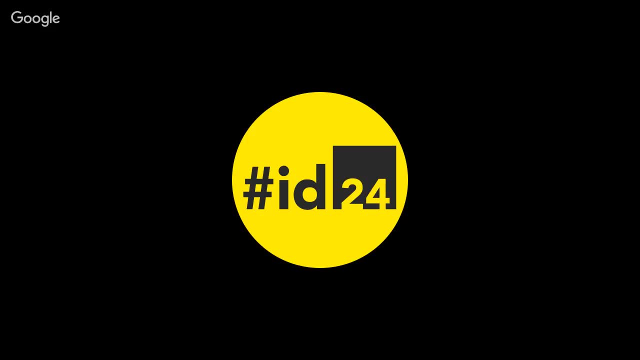 Hello and welcome back to Inclusive Design 24, brought to you in partnership with Barclays Access, the Paciello Group, Intopia, Microsoft Edge and Open Access Technologies. Don't forget, you can subscribe to Inclusive Design 24 on YouTube by visiting youtubecom slash Inclusive. 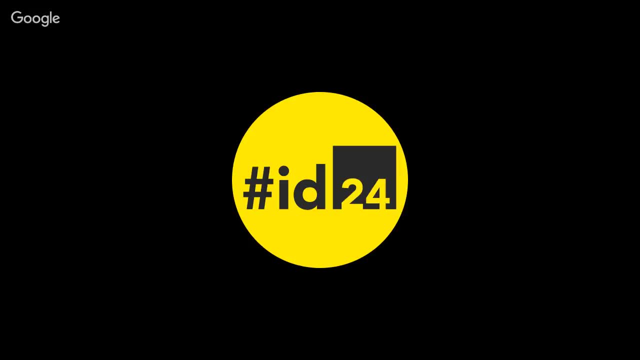 Design 24 and hitting the subscribe button. Don't forget to follow ID24Conf on Twitter and if you have any questions for the presenters, tweet them using the ID24 hashtag and we'll ask them at the end of the session. We now have Sarah Pulis and Andrew Art talking about using cognitive walkthroughs to better 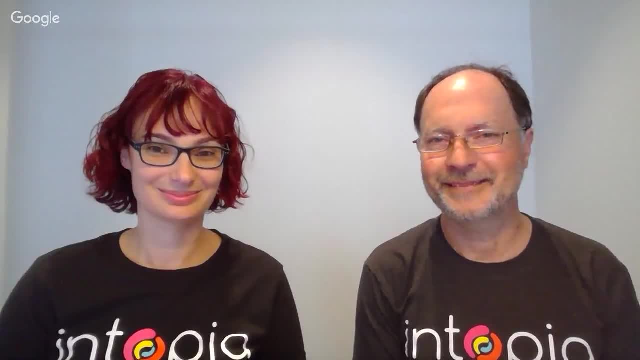 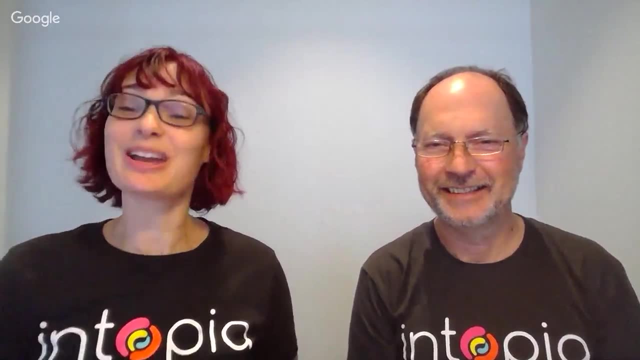 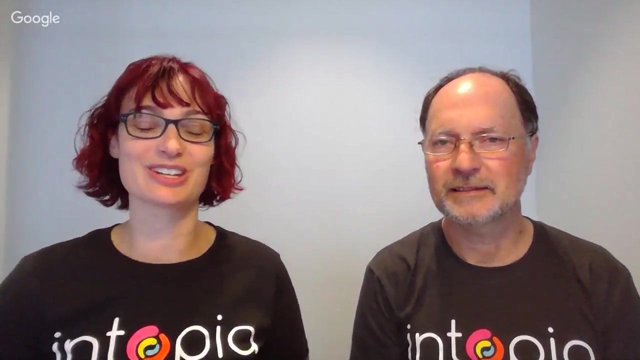 review designs for accessibility. So over to you, Sarah and Andrew. Thank you, Hi everyone. We thought we'd start by showing our faces, so it's nice to know who you're talking to. We're delighted today to join everyone who's watching now and later on from all around. 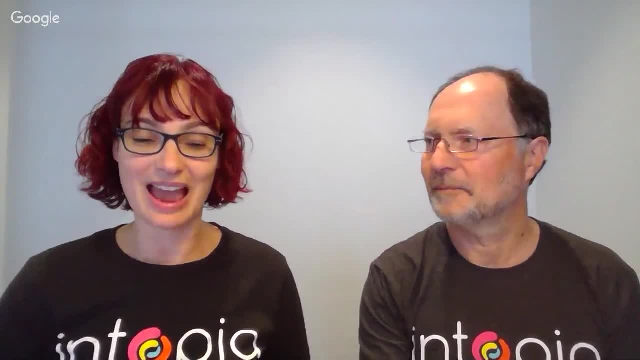 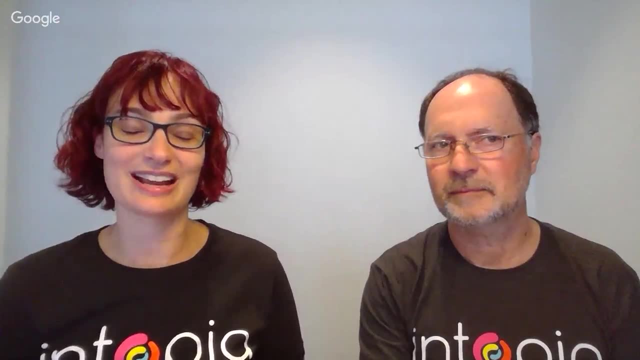 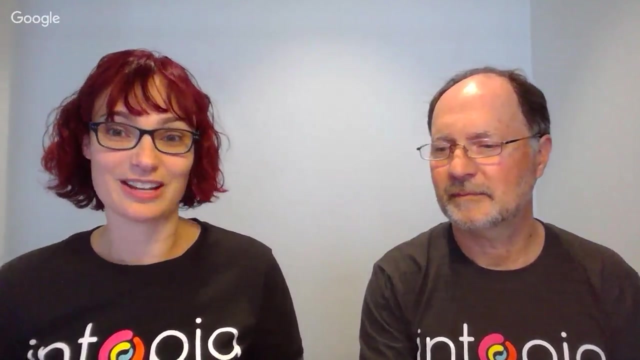 the world, sharing something that we have, I guess, come across when we've been working with clients and using this particular cognitive walkthrough technique to actually help to review your designs. I'm Sarah. I am one of the co-founders of Intopia. 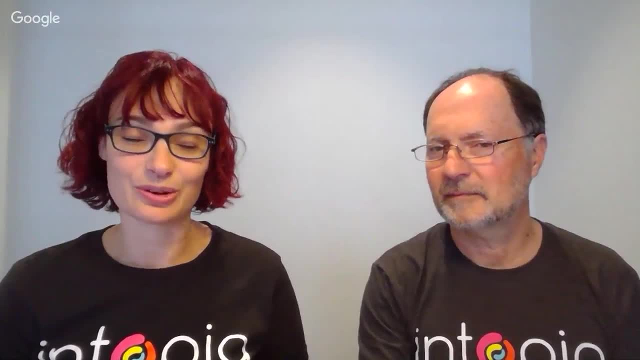 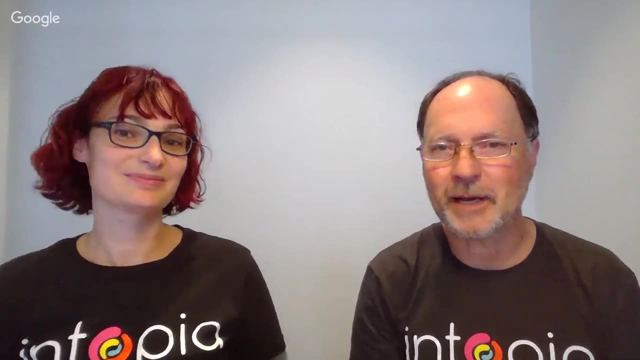 Hi, And we're delighted to also be able to support ID24 as one of its sponsors. Hi, I'm Andrew. I've done a few of these in the past, but this is the first time I've done a joint presentation. Sarah, I've done a couple of these lately and it tends to work quite well having two. 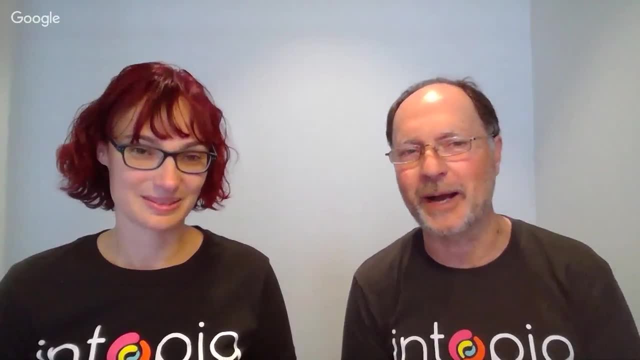 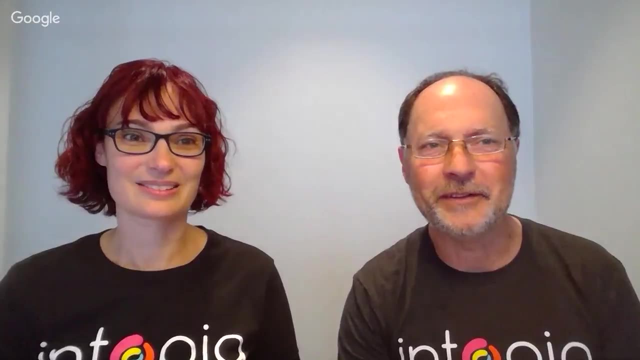 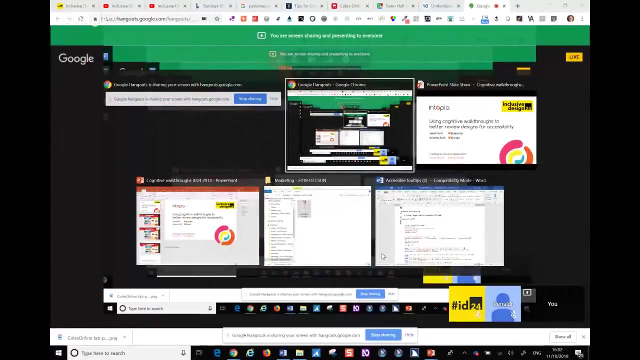 different voices talking about a topic that keeps everybody awake, particularly if you're listening in a non-waking time zone at the moment. So let's get underway with this and let's do a screen share, And there we go. Great, And I trust that you can now see our opening slide. 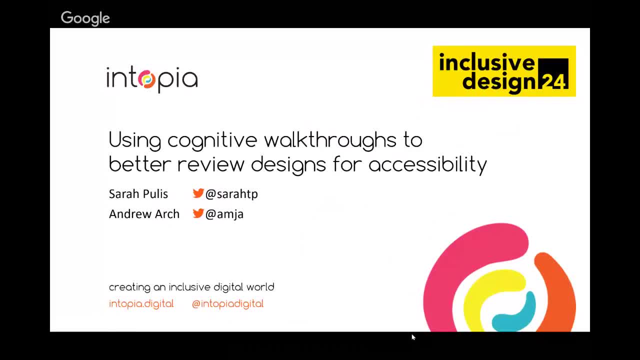 Can you please confirm that, Ian? Yes, we can see that. Great, Wonderful. If you were wanting to tweet us directly, my Twitter name is SarahTP, That's Sarah with an H, And I'm A-M-J-A, if you can understand the Australian accent. 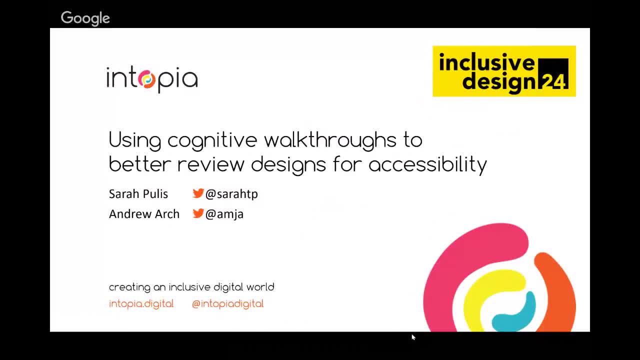 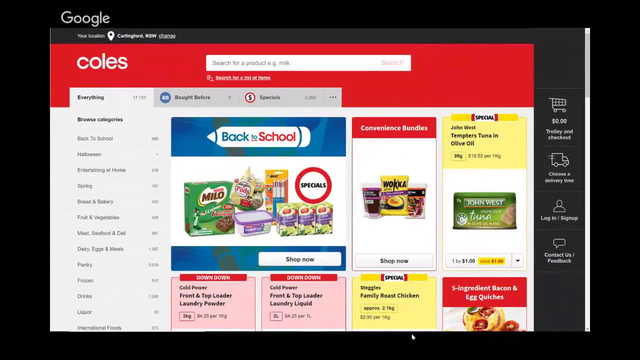 Okay, So I wanted to start off by actually sharing where this idea of using Cognitive Walkthroughs to better understand designs and how designs might work for your users. What we've got on the screen here is a screenshot of the Coles Online website. 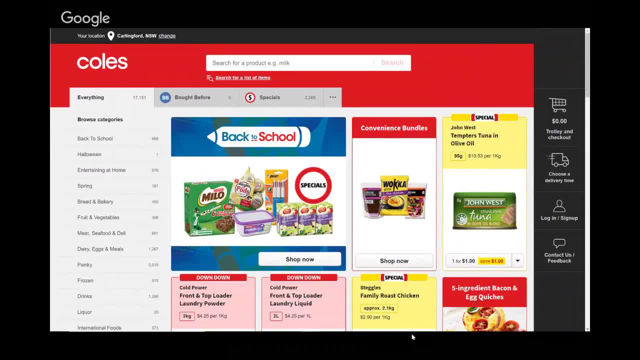 A little while ago, Coles Online actually did a complete redesign and build of the Cognitive Walkthroughs website. So in Australia this is one of our major supermarkets where you can buy our products online. They actually built this with accessibility front of mind. 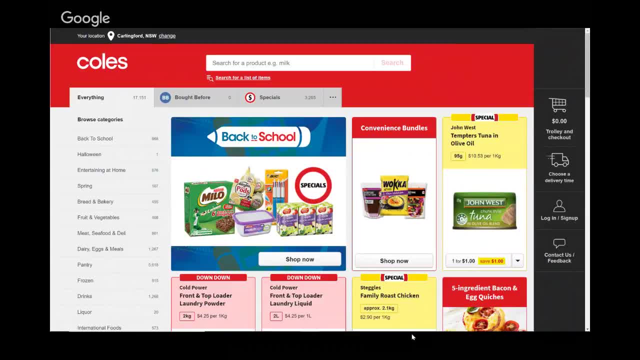 It was one of their core goals, their core principles, and they did have an accessibility specialist helping them with it as well. I actually came in towards the end of this to do a assessment against WCAG- the Web Content Accessibility Guidelines- to give them a report of how compliant it was. 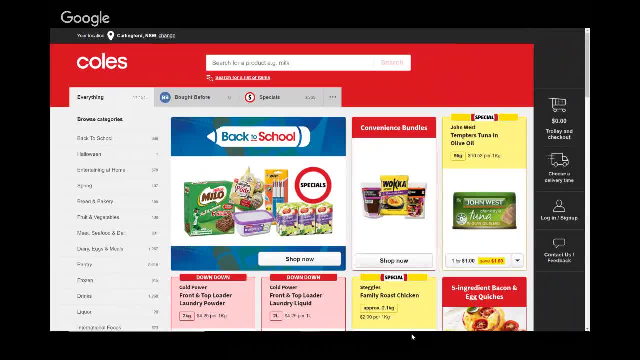 How compliant it was against each of the success criteria, And so I started to do that. We follow the WCAG EM, so the evaluation methodology where you create a sample set of pages based on unique pages templates, making sure that they're all pages that are within a process. 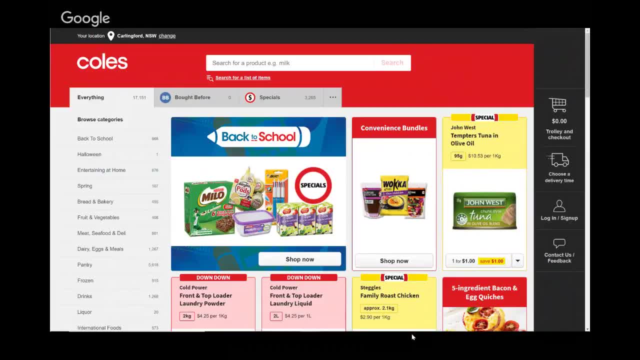 and then conducted the usual review against each of the success criteria. And as I was looking at this and testing it, particularly for keyboard accessibility, so making sure it could be used and accessed with a keyboard- I went actually it passes keyboard accessibility. 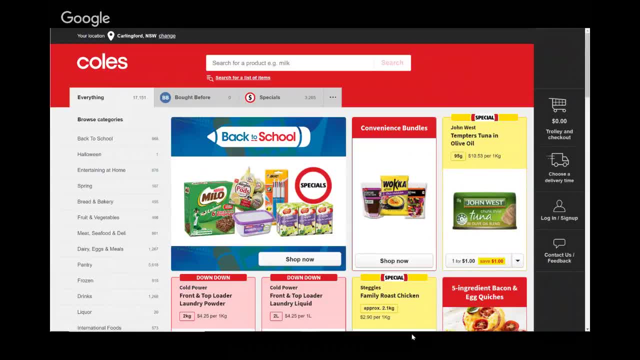 It can be used with a keyboard. The focus order is good. as I tab through everything, It sort of makes sense. But then I started to actually think about what task a user would be doing on this site. And usually what they do is they come in the site. 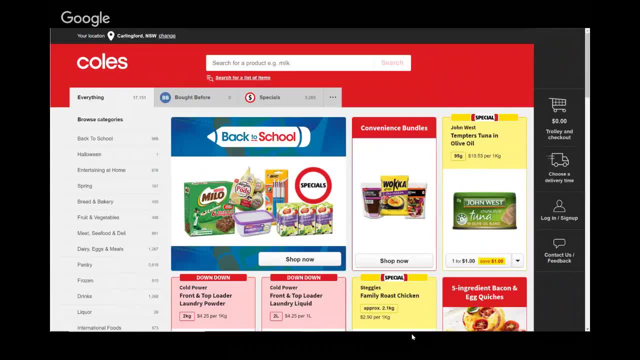 First of all, they'd have to log in if they had an account already. Once they've done that, they start to add items to their cart And then go to Trolley and Checkout. So I went: gee, there's the Trolley and Checkout is on the right-hand side. 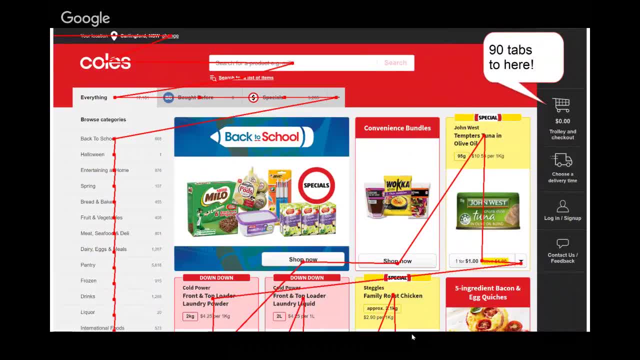 So at the top we've got sort of our standard bar menu, you know, logo, search field, what have you? We've got a few very little navigation, everything bought before and specials. We've got a whole lot of categories that we can go through. 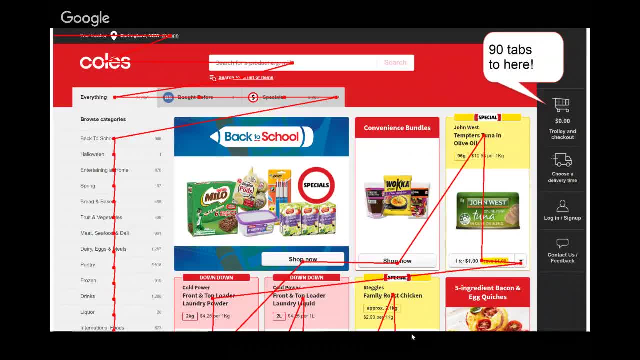 And then we've got our main content area, which has a lot of product tiles, And I thought: well, how many tabs would someone have I have to press in order to get to the Trolley and Checkout button, which is pretty important. 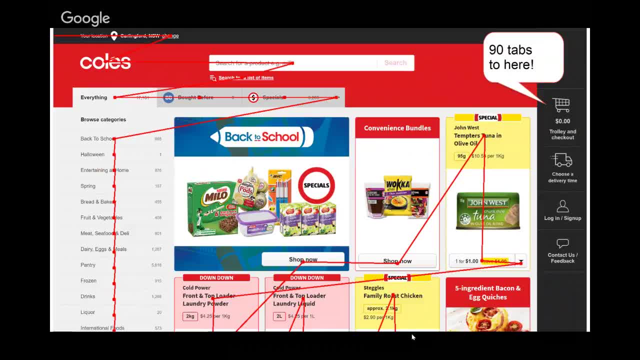 when you put things into your cart and want to check out. There's actually 90 tabs between the very top of the screen. so Cole's logo going through all of that, that banner area, those browse categories, all of those product tiles. 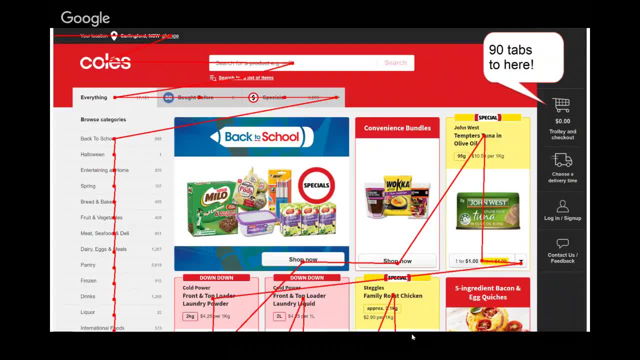 And then, finally, I get to that bar which is visually on the right-hand side that says Trolley and Checkout. It's like you can use the Trolley and Checkout button and then enable the app to go through that, And then you can use the Trolley and Checkout button to go through that part of the page. 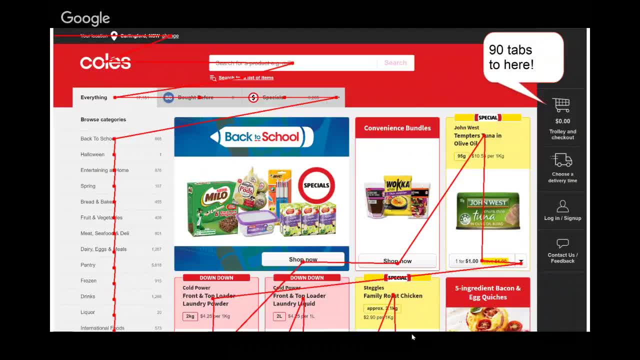 and just pick a little piece of it, which you don't always see in the first page. But if you're just going to go through it, just make a couple of clicks and it will let you know where you want to go. And you can also, as you can see in the right-hand side, you can go through this and it's very. 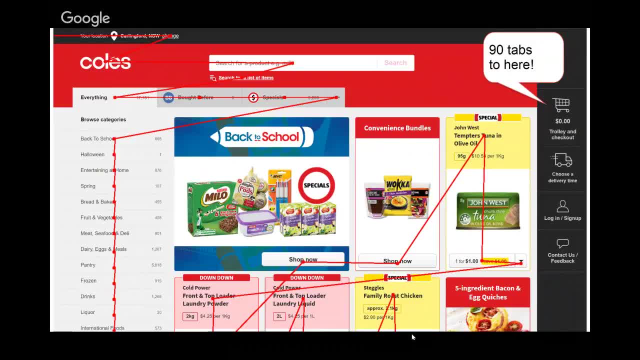 simple, And you can also use the Trolley and Checkout to do that. And that's all I wanted to talk about. Thanks for your time. So I fed this back to Coles and they're like: yeah, we agree that that's a bit of a problem. 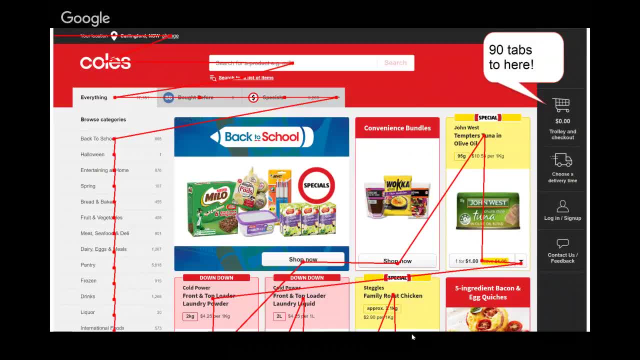 But because this site was already built, we couldn't change the order of the. you know the order of content essentially. So bringing that trolley and checkout and those other items earlier on, it would just be too much redevelopment. And so what they did was they actually implemented some skip links. 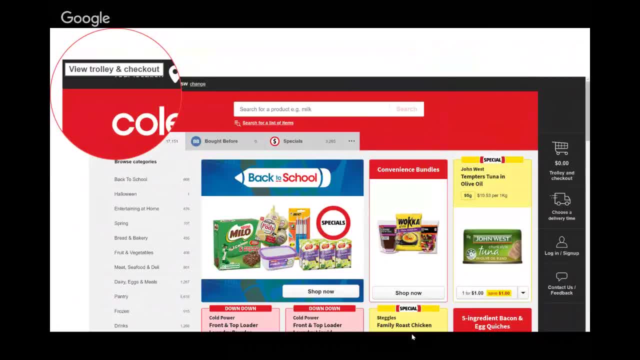 So on the site currently you've got your standard, you know, skip to main content. but they also added a view to trolley and checkout link, as you can see on the slides now, And there's also another one that is actually a skip to login. 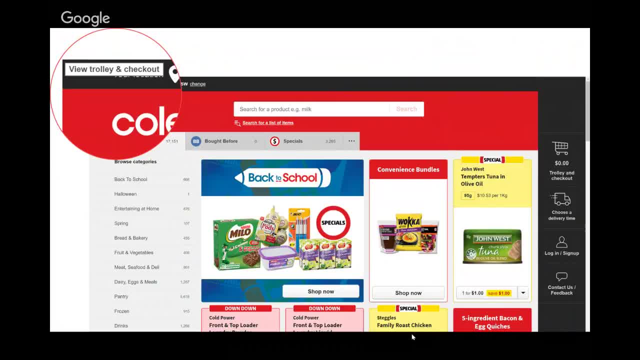 But it started me thinking how can we better look at sort of what the task, you know the task that someone is trying to complete, as opposed to what usually happens in a standard WCAG review, which is we might have all the pages that were in a task or process according. 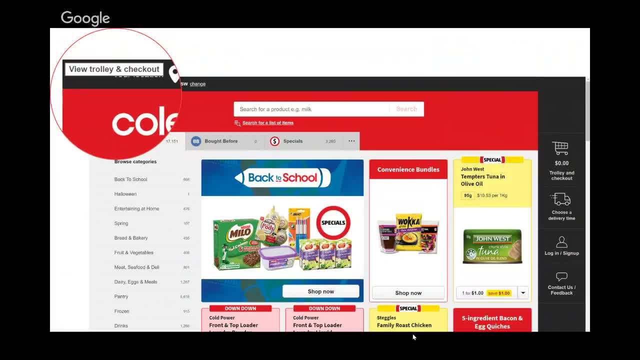 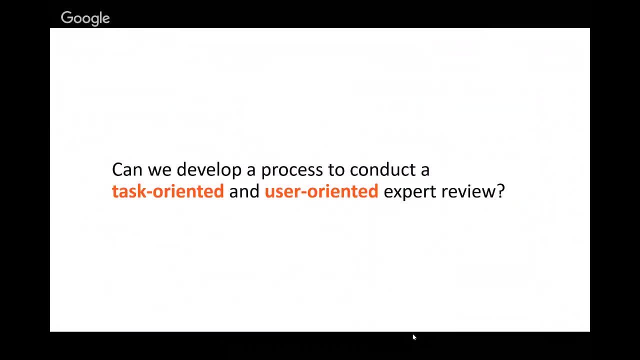 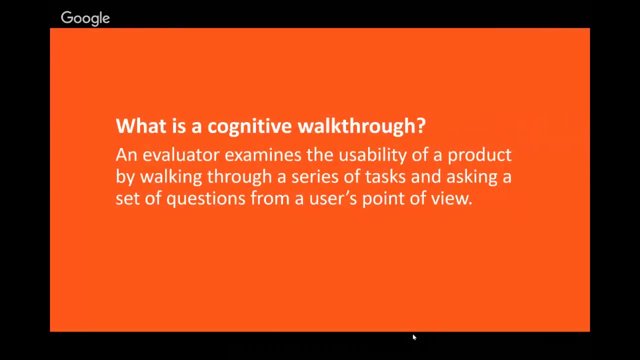 to our nice evaluation methodology guidance, but we're not always focused on that task, what the user is going to do. So the crux of that question was: can we develop a process to conduct a task oriented and user oriented expert review? So the UX technique for this is using a cognitive walkthrough. 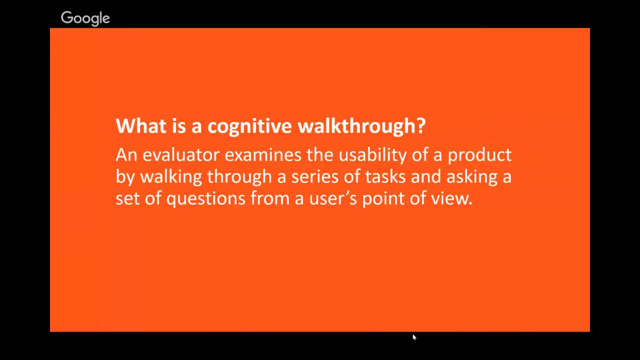 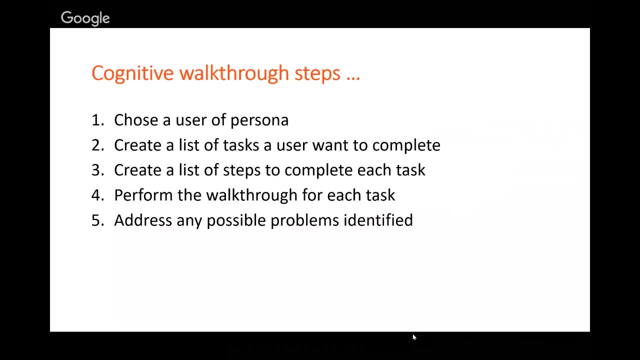 It's task specific, it's driven by usability and you actually walk through. can you actually complete all these tasks and ask a series of questions from the user's point of view, The different steps that you undertake? typically, you'd be choosing a persona you know in. 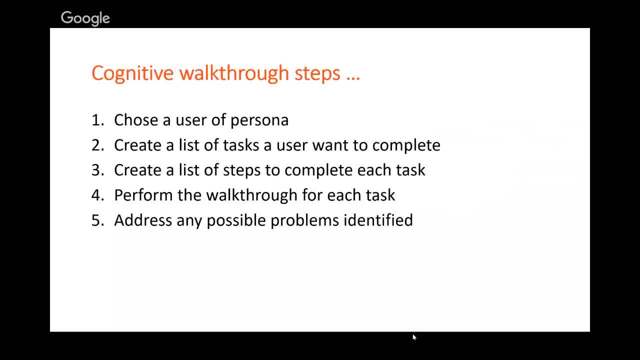 the case of accessibility, we want different personas with different abilities so that we can step through with different assistive technologies, different adaptive strategies and so on. We would then create a list of tasks that the user is expected to complete, such as buying a block of chocolate, putting it in their cart and paying for it. creating a list. 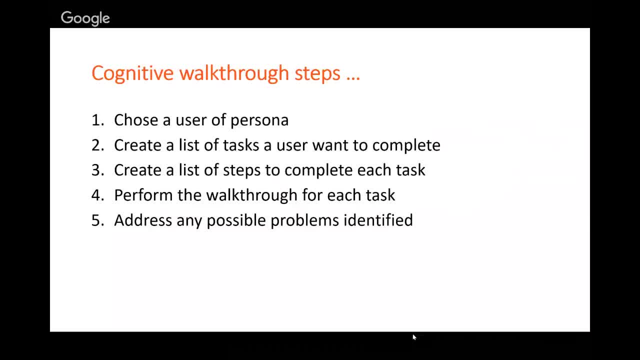 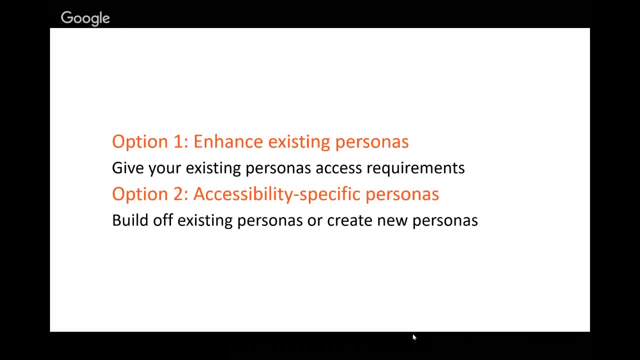 of steps to complete each task: performing the walkthrough for each task and identifying the issues and then addressing possible problems that have been identified. So step one: choose a persona. A couple of ways you can do this. You may have existing personas. 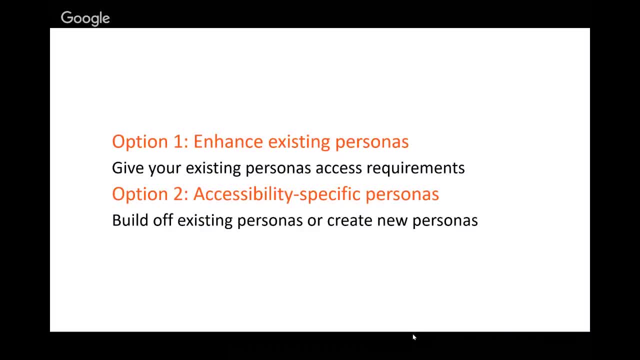 And you can give your existing personas some access requirements or, preferably you may have, you may create some accessibility specific personas, which is an easier way of making sure that you're covering all the needs of a different range of people with disability. But just adapting some specific personas is a very good way if you've already got those. 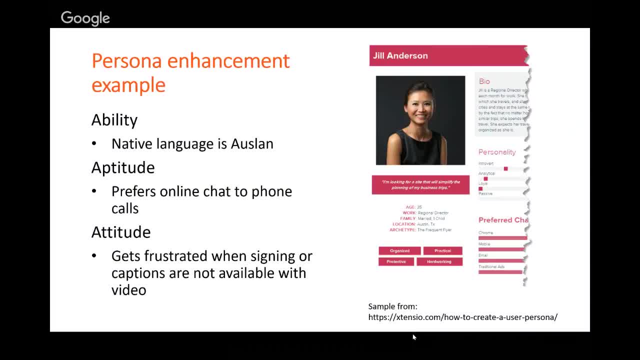 For instance, Jill Anderson here is the regional director. She's age 35. She's married with one child. What we were able to add to her was an ability. her native language is Auslan. She's highly deaf, completely deaf. 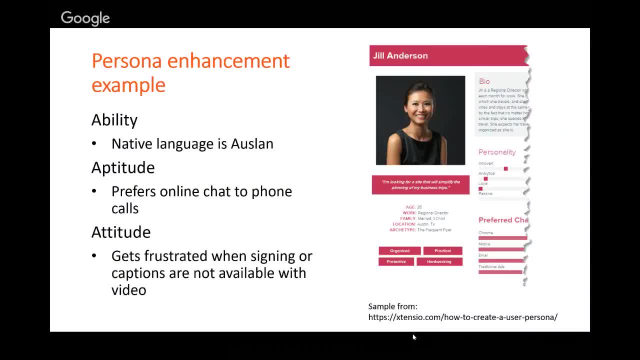 So she learned Auslan before she learned English or Australian. She prefers online chat to phone calls. Obviously she has difficulty hearing and she gets frustrated when signing or captions are not available on the video. So a good persona should talk to you. 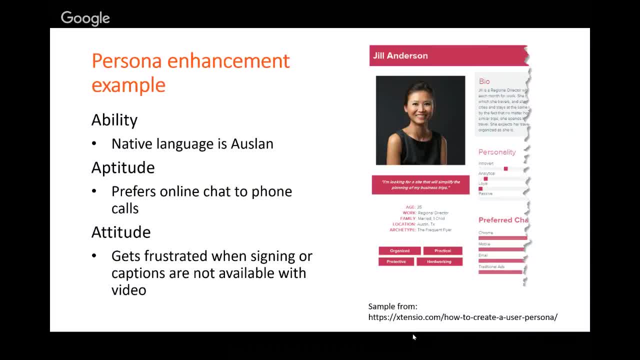 Talk about the persona's ability, any assistive technology they might use or require in certain circumstances. The effect their ability has on the digital experience, and that's often known as aptitude. And then their motivation, their emotion, their risk tolerance, how likely they are. 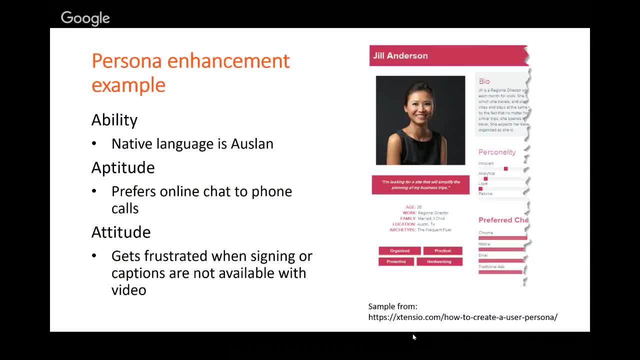 to persist even when things get difficult is their attitude towards completing the task or their attitude towards using their technology to complete a task, And the ability, aptitude and attitude come from the book A Web for Everyone. A Web for Everyone actually has some accessibility-specific personas that you can actually have a look. 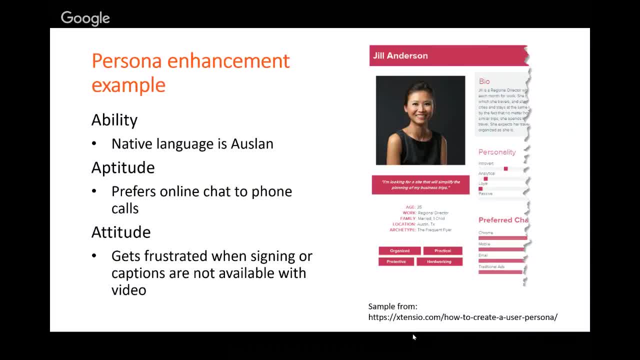 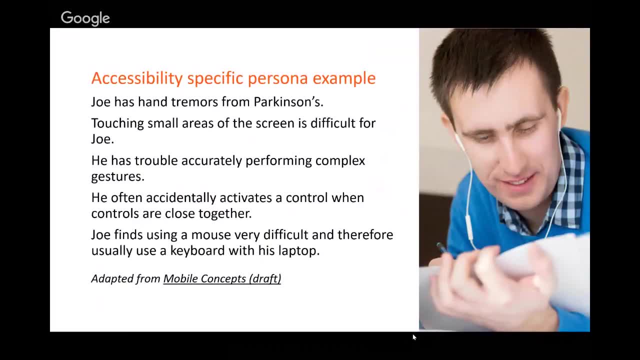 at online, But they phrase things as the ability, the aptitude and the attitude, So an accessibility-specific persona. we've got Joe here. Joe has hand tremors from Parkinson's. He touches finds touching small areas of the screen is difficult. 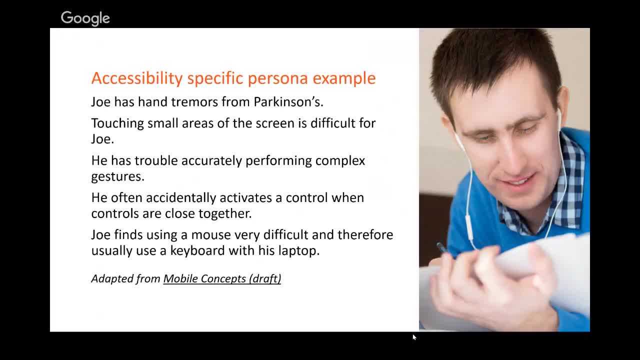 So he's got a hand tremor. He's got a hand tremor. The screen is difficult because he can't control that tremor. He has trouble accurately performing complex gestures. He often accidentally activates a control when the controls are too close together. 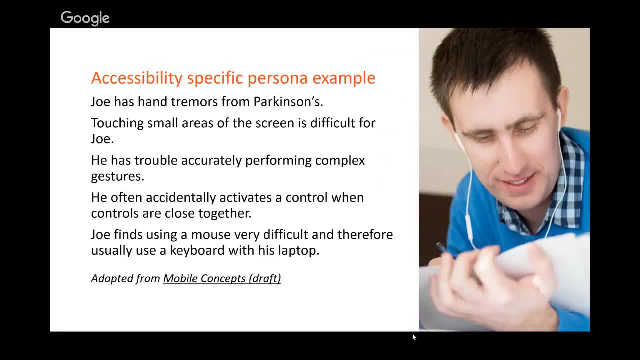 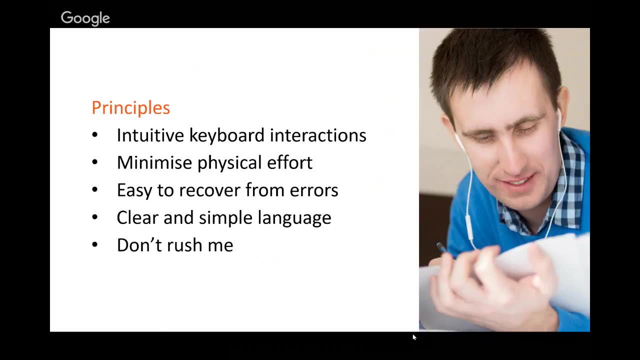 He finds using a mouse difficult and therefore regularly just uses a keyboard to navigate, even though he can use a mouse, but he finds it really difficult. So the principles behind what we want to achieve, What we want to achieve with our cognitive walkthrough for Joe is: do we have intuitive 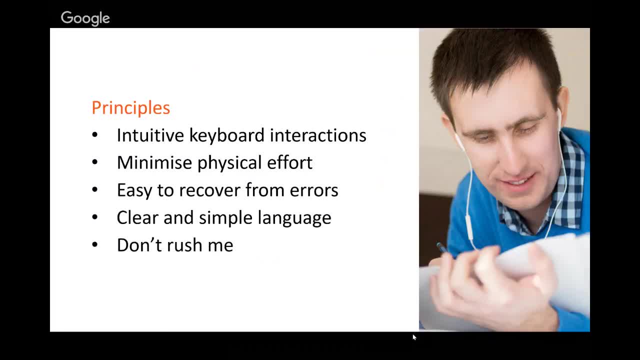 keyboard interactions. Are they the commonly used keyboard interactions? And if we come across a dropdown, for instance, yes, there's a keyboard command- alt down arrow- to reveal the list of options behind that dropdown list, but our finding is that most people don't know it. 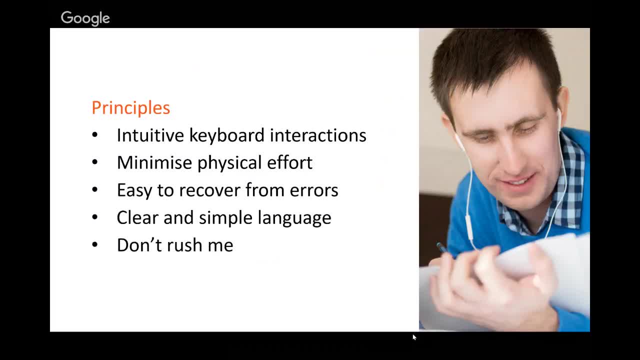 Occasionally you come across somebody who does, but most keyboard users aren't aware of that. We want to minimize the focus. We want to minimize the focus. We want to minimize the physical effort for Joe. We want to make it easier for him to complete a form. 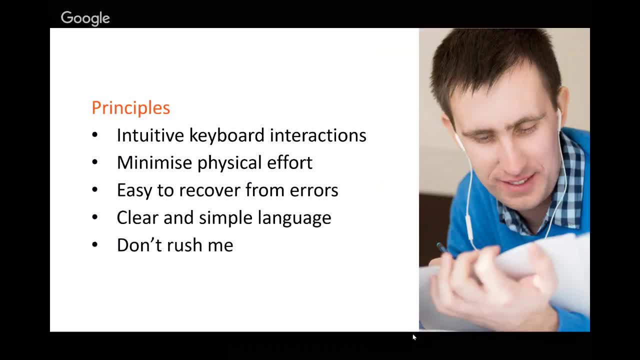 He's obviously going to have some trouble typing with some of the issues that he's got, So auto-complete, for instance, would help him complete a form, and an optimal path and focus order is obviously going to make life easier for him. Can we make it easy to recover from errors? 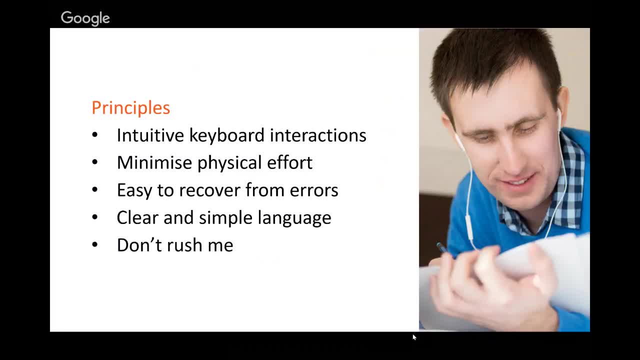 Just obvious because we want to minimize the effort. Are we using clear and simple language? Will Joe and other people understand the instructions that they're given to fill in that form or put things into their cart, And are the labels intuitive? Have we got clear labels for all our text forms or the calls to action that we're expecting? 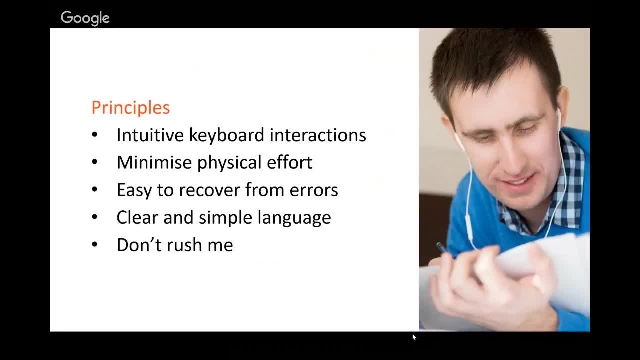 Joe and other people to follow. And finally, don't rush me. I mean, Joe's probably going to be slower to use the computer than somebody who can use a mouse and a keyboard because he has to move through using the computer. So we're going to have to make sure that he's using the computer. 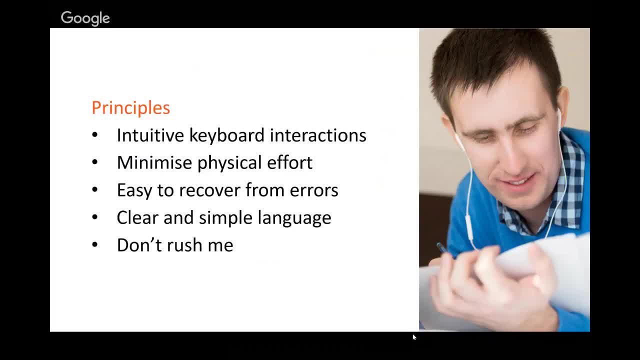 We're going to have to make sure that he's using the computer. We're going to have to make sure that he's using the keyboard to activate everything. So we want to make sure that Joe isn't going to be timed out and that he's got save and 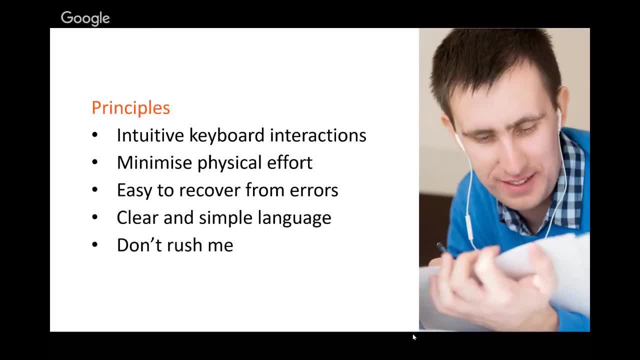 continue options and things like that as he's progressing through an activity. I think these principles are quite important When you're using the persona to conduct the cognitive walkthrough which we'll get to soon. if someone is not as familiar with how different people navigate, interact the different. 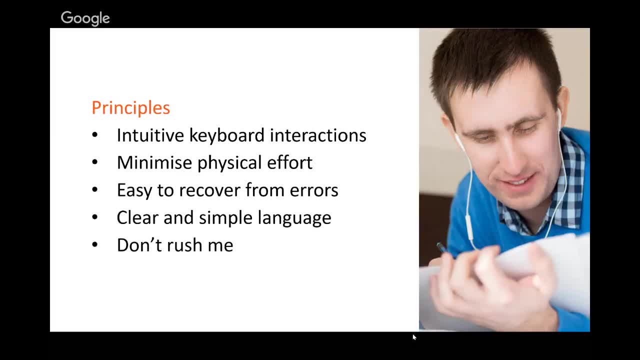 technologies they use. These principles are core to being able to better conduct that walkthrough. So the things to keep in mind as we conduct the cognitive walkthrough: are the keyboard interactions intuitive? What is the physical effort like for someone like Joe? So this is really great for, particularly if you're using this particular technique with 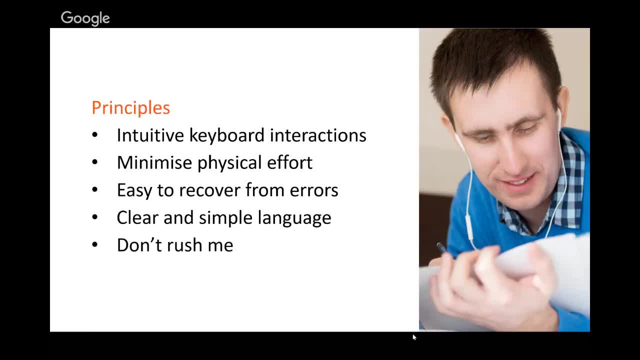 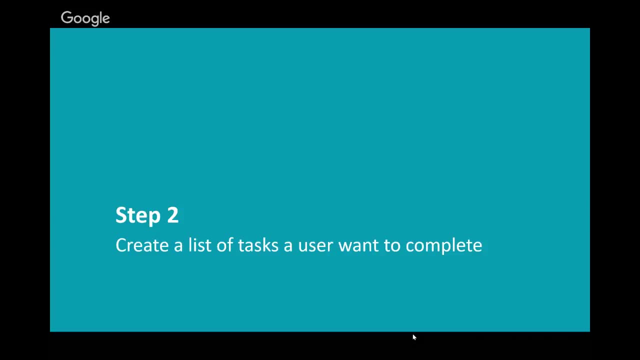 people who are newer to the diversity space. It really sort of drives home some of those things that they need to think about as the task is completed. It might also be worth mentioning. I guess there's a lot of negative press about personas. 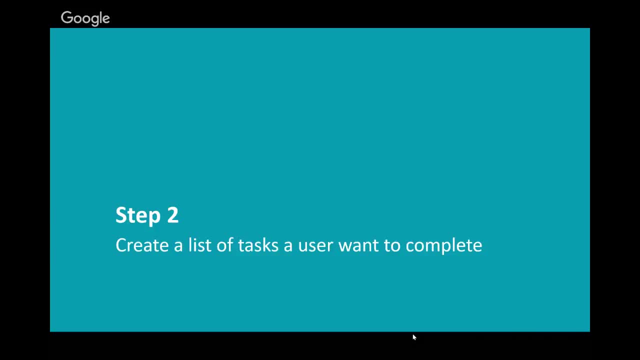 so to speak, that personas are often. they try to be representative, but everyone is different and you're trying to sort of make a persona that covers a whole lot of things or a number of personas. A lot of organisations do use them and sometimes some of that gets lost in the mix. 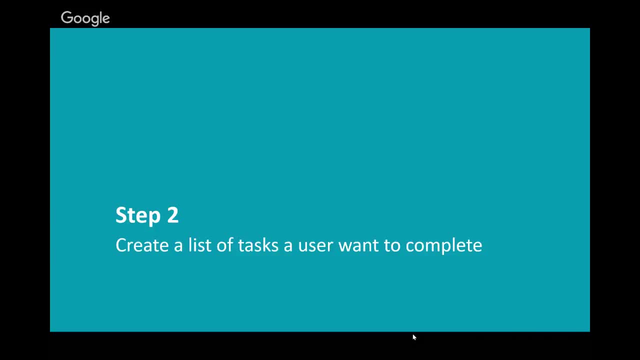 I think, though, for cognitive walkthroughs they're ideal, in the sense of we can use them to, I guess, get some of those different abilities and actually walk in the shoes of that particular user And if you're still planning to get real users in to do some testing doing some of these, 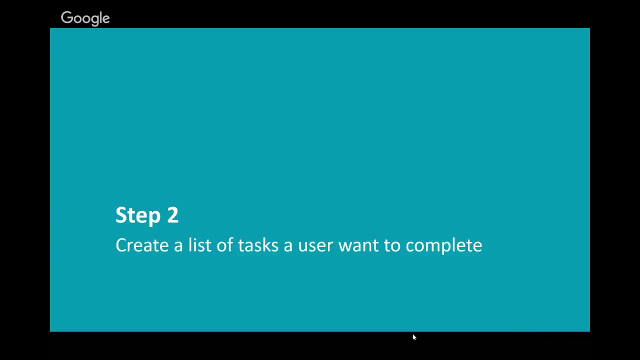 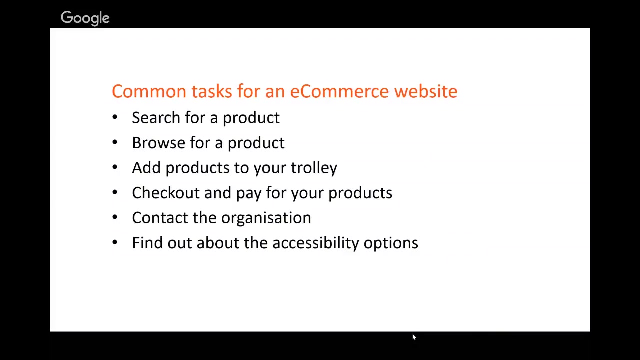 cognitive walkthroughs can eliminate those barriers that mean you're not wasting your time and their time when they do So. the next step is to create a list of tasks that we want the user to complete. For an e-commerce site, for instance. we might have searched for the product might be browsed. 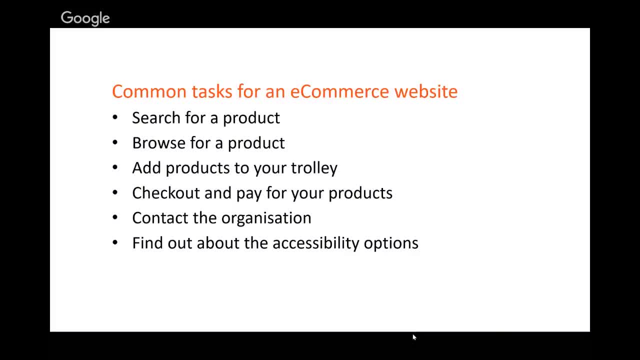 for the product If we've got all the products on the screen. like Cole's had a series of categories- I think bakery was one and you might be looking for Christmas cake- Add products to your trolley, go to the checkout and pay for your products. 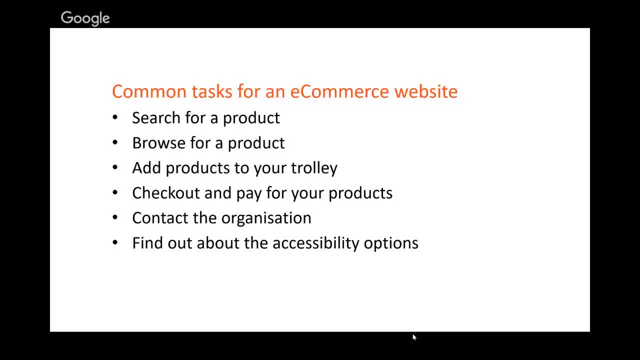 You might need to contact the organisation if you've got any issues, And a lot of people with disabilities actually do want to check about what the accessibility options might be, and it might be beyond the digital product, such as delivery options going in store, is it an accessible store? and things like that. 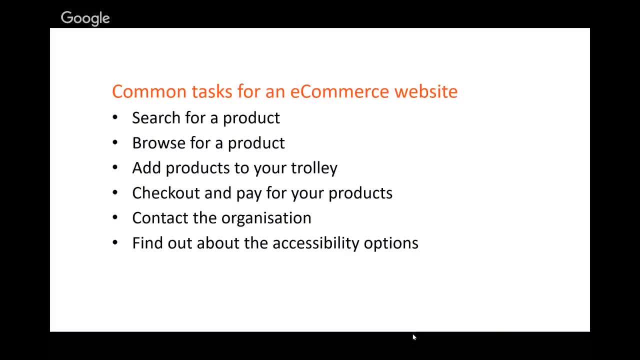 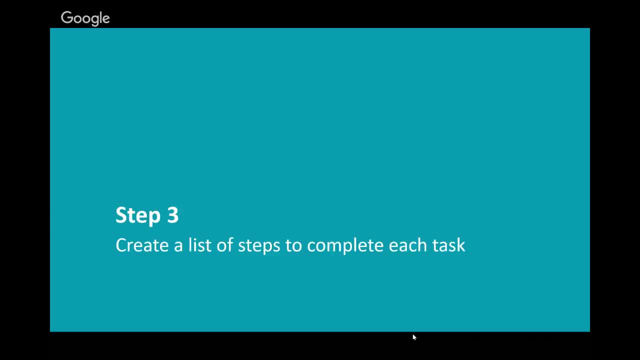 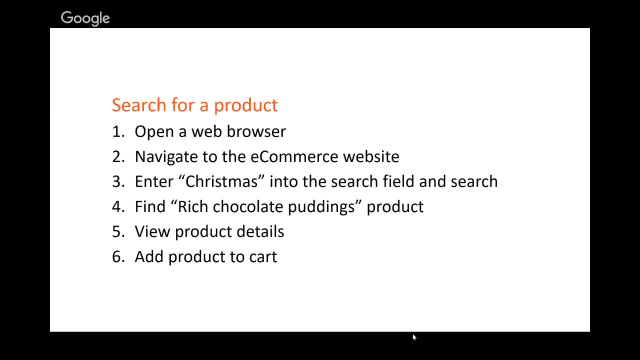 So there's a whole lot of other things, apart from the e-commerce task itself, that they may want to access successfully Create a list of the steps required to complete that task. So, in this case, open the browser, navigate to the e-commerce website of the organisation. 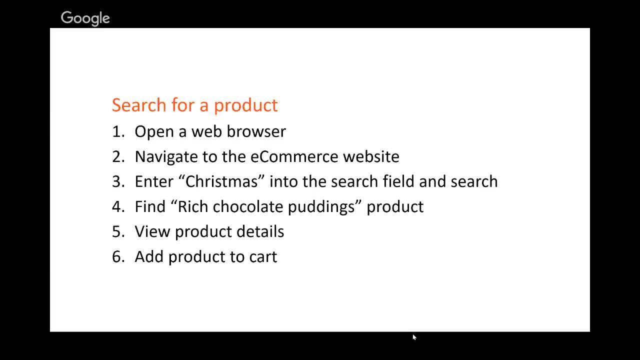 You might want to be putting Christmas into the search field. find the rich chocolate puddings product, check the details of it- Are there enough calories there for you for Christmas day? And then add the product to the cart and check out. So they might be the typical tasks to purchase that. 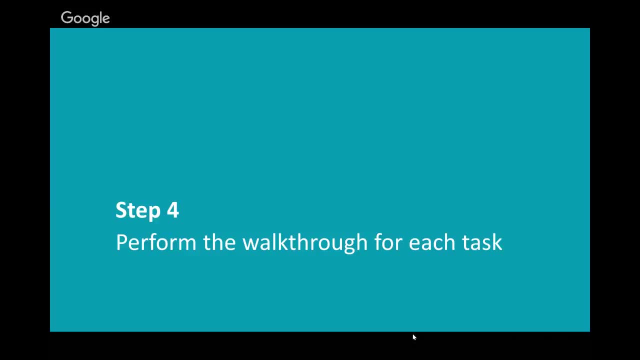 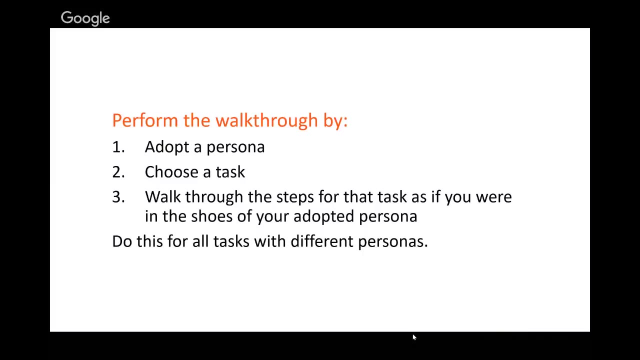 And then we want to perform the walkthrough. So, when we perform the walkthrough, the first thing is we adopt one of our personas. So, as I mentioned, there's quite a number of accessibility related personas that you can actually use online. So, with everyone I mentioned, they've got eight different personas. 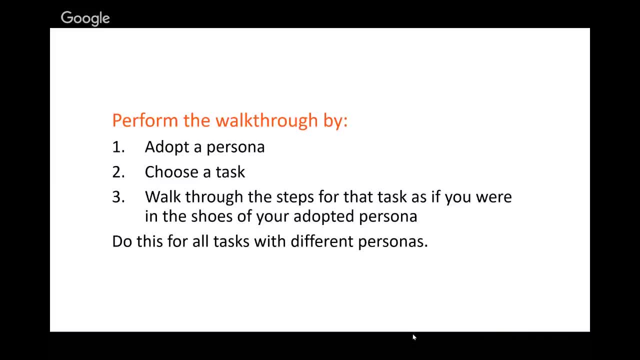 GovUK also has some really great personas. I think there's six of them from memory. Barclays Bank is another one. So if you're just starting out using these or wanted to borrow from someone else, there's plenty of plenty out there for you to start with. 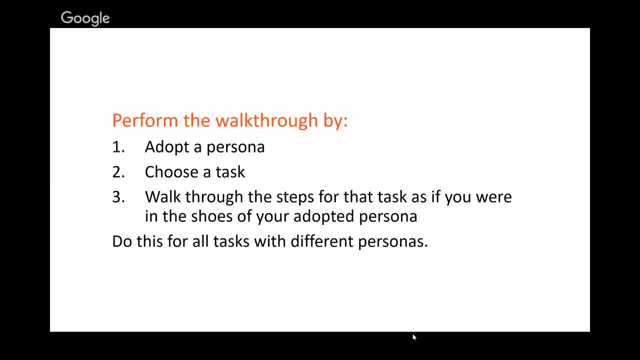 GovUK, in particular, their personas also have a few of those tips down the bottom about how to design for that particular persona And that sort of aligns a little bit with what you're looking for. Yeah, GovUK, in particular, their personas also have a few of those tips down the bottom about. 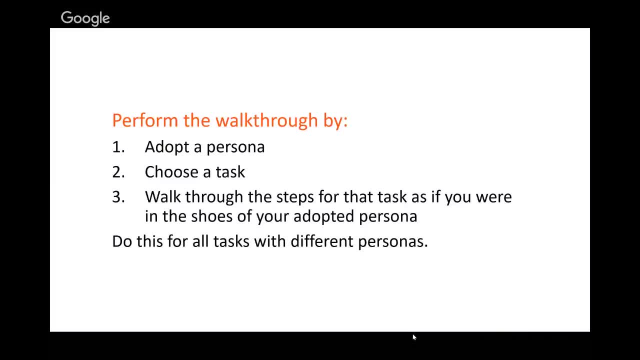 how to design for that particular persona And that sort of aligns a little bit with what you saw before in our example- accessibility persona- with those principles. So that's a great starting point for you. So, essentially, you pick up the persona card, you choose one of those tasks that you identified. 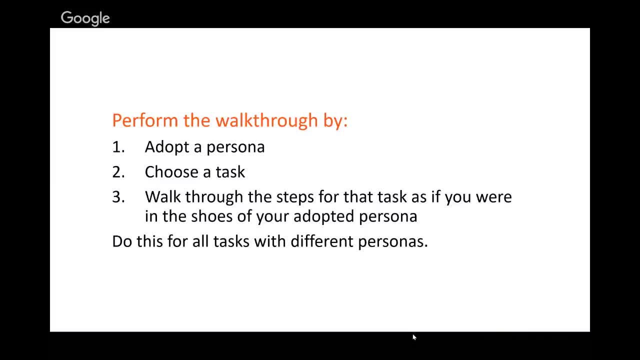 in step two. Often, those tasks are things that you probably already identify as part of your general UX process, And then you walk through the steps that we identified in step three for that task as if you were in the show. So, in Joe's case, get rid of your mouse, because it's too easy to reach for it when you're. 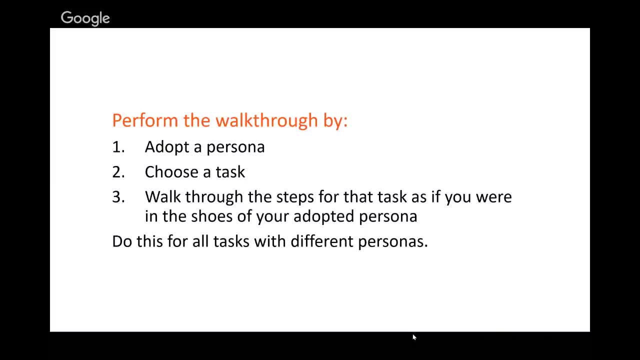 trying to get walk through something and just use the keyboard. My experience has been working with developers and designers that they just cannot avoid putting their hand back on the mouse to complete a task. So I've had to unplug the mouse many times or remove it or cover up the touchpad. 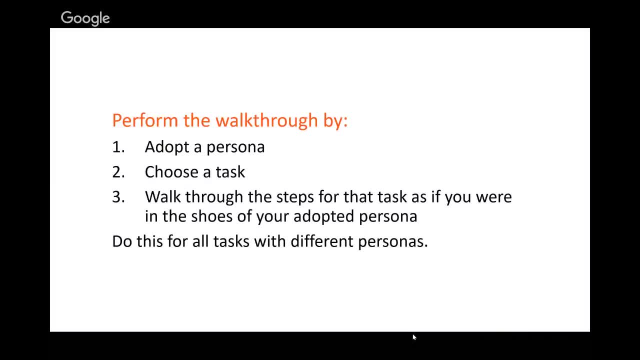 GovUK in particular. their personas also have a few of those tips down the bottom about how to design for that particular persona, or because it can be done once the website is developed, as Andrew said, but it also can be done at the design stage. 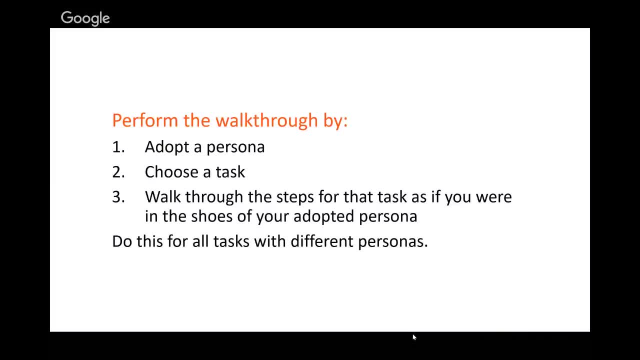 So if we were looking, for instance, at Joe and keyboard interaction on some visual designs, let's say you can actually be walking through and looking at what are your interactive items on the page. how many tabs is it to go through? is the keyboard interaction clear? 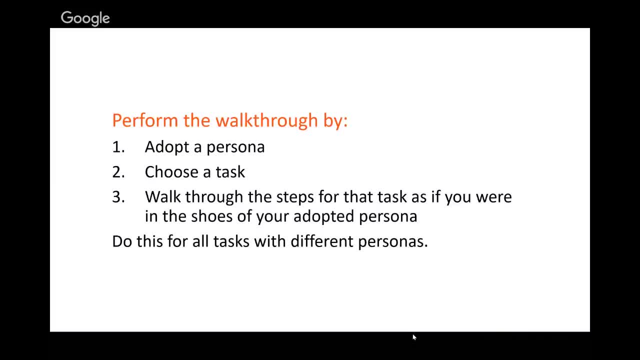 So have you, for instance, used standard components, that that keyboard interaction is clear? Or if you've created a custom component, perhaps you need to actually make sure that at that design stage you've identified what the keyboard interaction should be, so that that can be then passed off to the developers. 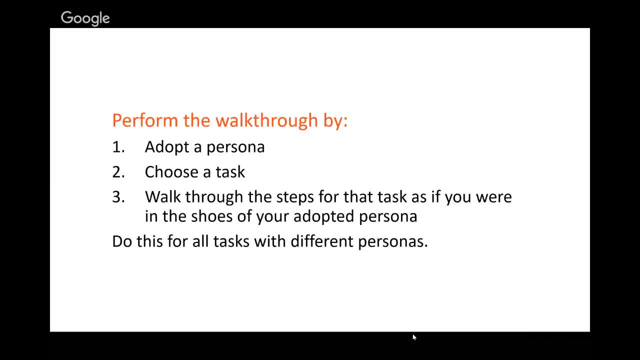 It's quite clear, you know what you want that experience to be and it also cuts down on rework. So if that's not defined or is not clear between the designer and the developer, that can add, you know, a lot of extra time if you find you know. 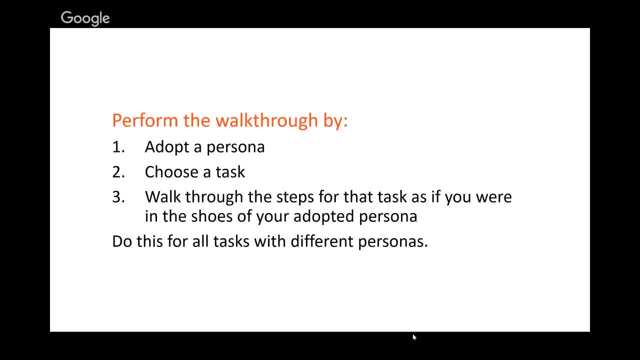 later on that it actually is not working as you wanted or anticipated that it should. So this is ideal for both of those situations And if they've done a cognitive walkthrough of the mockups of that Coles shopping site, they may have realized early on. 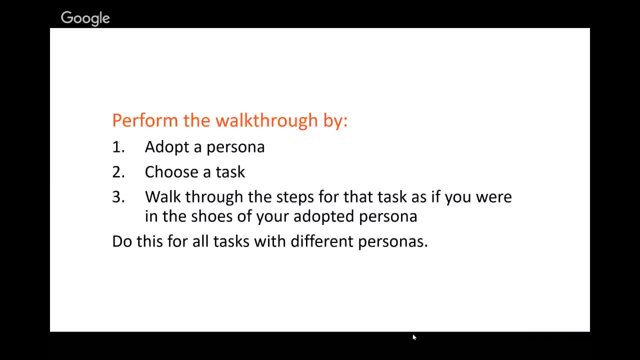 at the design stage that, hey, we want people to be able to get to the login screen and the checkout much more easily than Joe, whilst the way Sarah walked through it when she was doing her analysis And that could have been part of the specification. 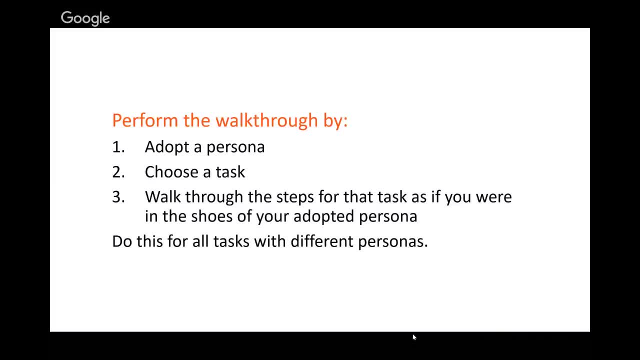 that got passed on to the developer saying: yes, this is sitting on the right-hand side, So it's typically late in the order of things on the page. But hey, we want people to be able to get to it quickly. We want to have a skip to that shopping cart as part of the opening screen. 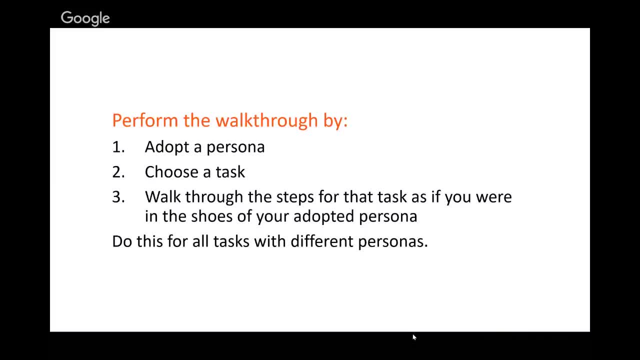 even though non-keyboard users don't need it. We want to make it obvious to keyboard-only users Or alternately, when you think about it, a lot of the time you see cart buttons actually in the banner. So although it's positioned on the right-hand side, 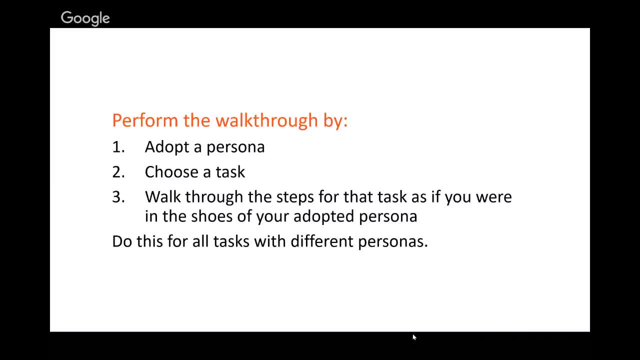 we may actually say you go through the banner items and then actually the next lot of items is that trolley and checkout, delivery time, login and so on, And then we move on to the main content area. so those browse categories and what have you. 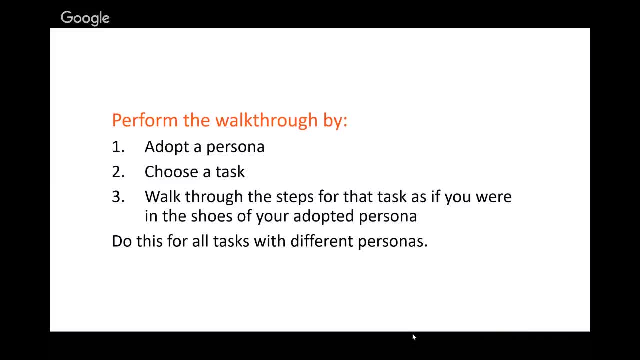 But by the time that I'd picked this up, it was sort of too late to do any major changes like that, And so that's why the skip link, I think, was implemented, And that's really where the crux of this presentation came from. 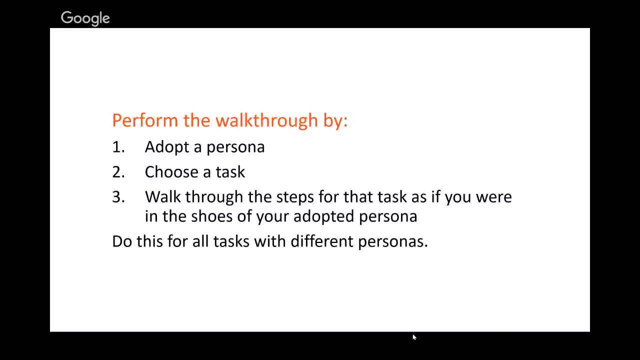 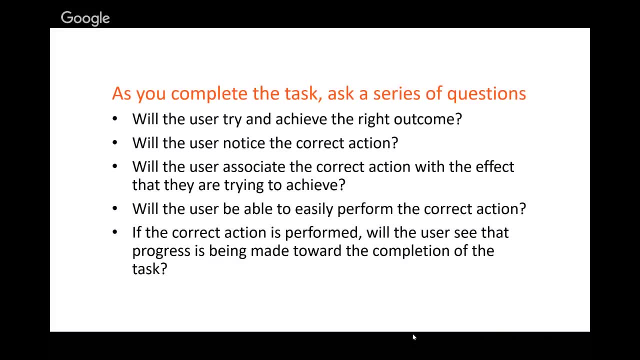 was thinking about how we could pick up those type of issues a lot earlier. So one of the key things when you conduct a cognitive walkthrough is to ask yourself a series of questions as you're moving through the walkthrough in the shoes of your particular persona. 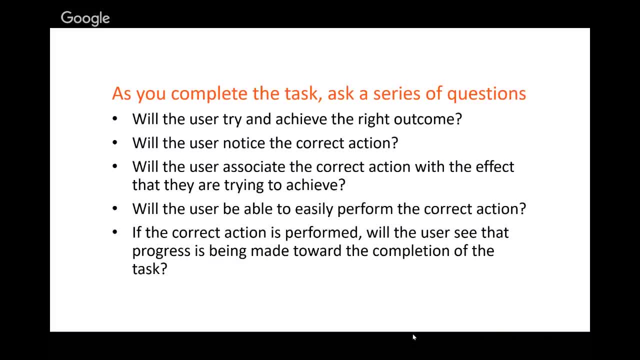 So this looks at: will it be obvious? Will it be obvious what a user needs to do? Can they actually do that or do that step, And will they know when it's done? And we've got five particular questions around this. The top four actually come from more a standard cognitive walkthrough process. 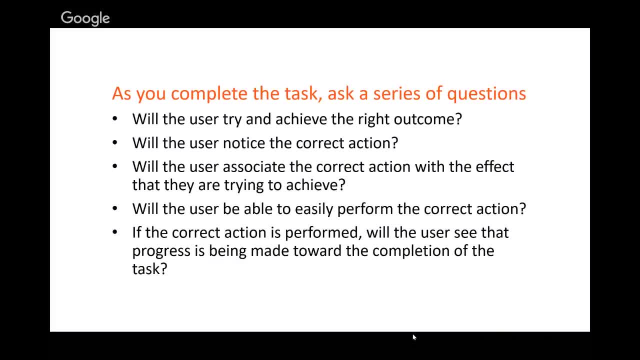 Oh no, actually the top three and the fifth one are the standard cognitive walkthrough process. We actually reordered these ones. The fourth one is something that we've added in specifically because we felt there was a gap from an accessibility standpoint. So let's walk through these and see how we go. 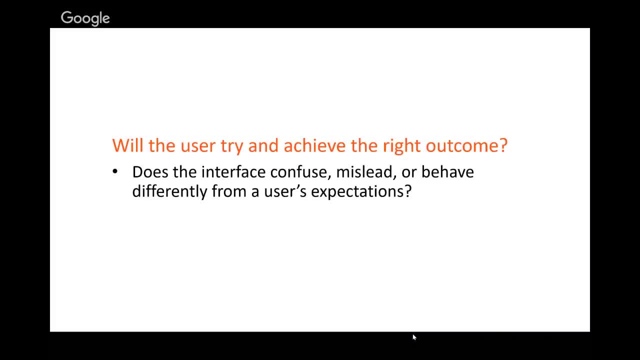 So will the user try and achieve the right outcome. Does the user know what to do at each step to achieve their goal? And an example of that is: how are you designing- maybe how you're designing- tabs on a page? Most users in our experience who are keyboard-only users, 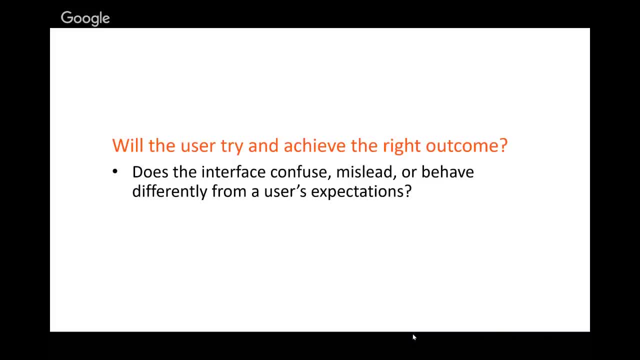 tab through the page to get to the interactive elements. The latest design- well, not just the latest, but current designs for tabs tend to have you tabbing to the tab, pressing a down arrow to open it and then continuing to tab or arrow through those. 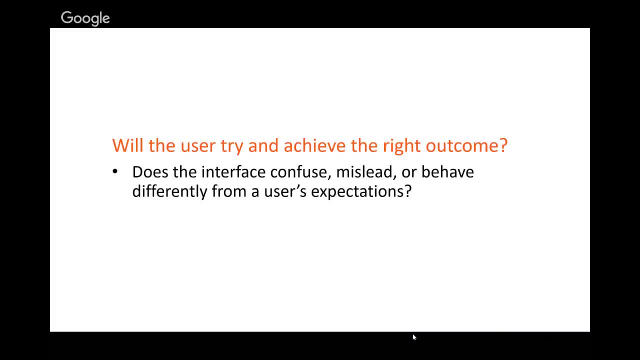 But, as I said, our experience is that many, many users are familiar with that new pattern, design pattern, and so they're tabbing and they're finding that they can't get to anything that they want to get to. So is the design going to be different? 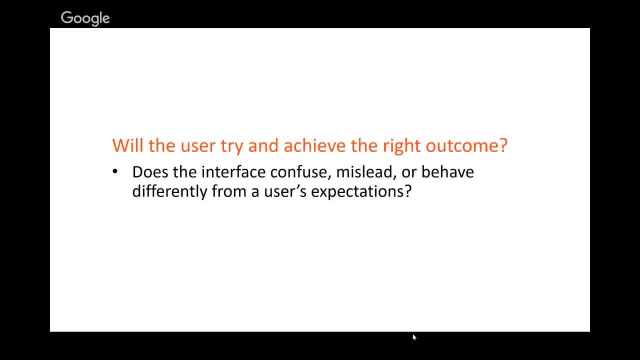 Is it going to expand? Is it going to behave differently from their expectations? Yes, there's a chicken and egg thing. At what stage do we introduce something new and expect users to be able to adopt it, But if we want them to be able to try and achieve the right outcome quickly, 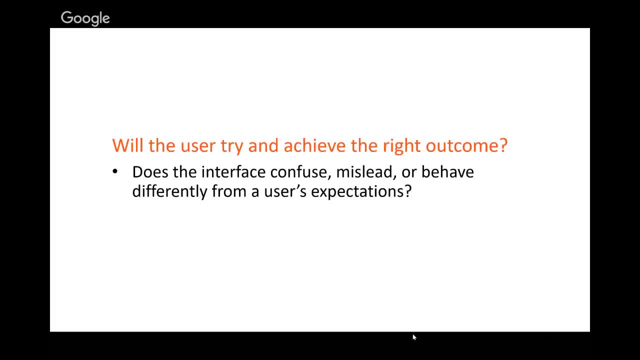 then maybe we're better off using the design patterns that they're familiar with from the last decade of their experience. So the next one is: will the user notice the correct action? So is it easily noticeable? Can I see it on the screen? Does it stand out? 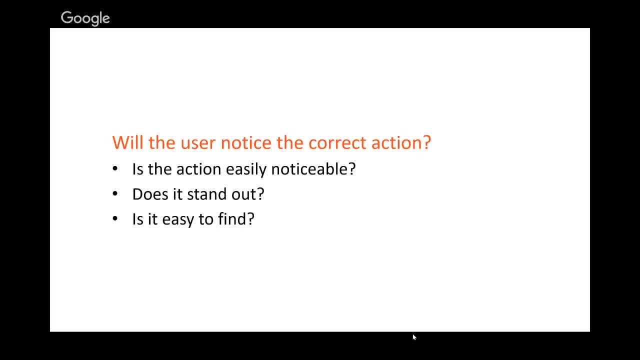 And is it easy to find. So again, depending on which persona we've got, these questions can play out in different ways. For instance, we're actually talking about chat and how a lot of the chat buttons are on the far right-hand side of the screen. 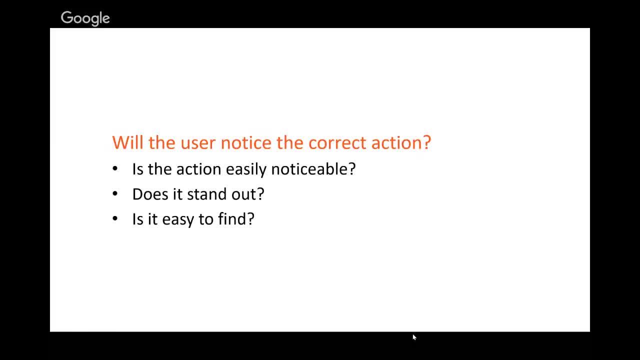 Sometimes, if you're, say, a screen magnifier user, or even you know other users that are focusing more on the centre of the screen, you might actually miss that button to the far right-hand side, particularly if you've got a website where it's sort of you know, centre-aligned. 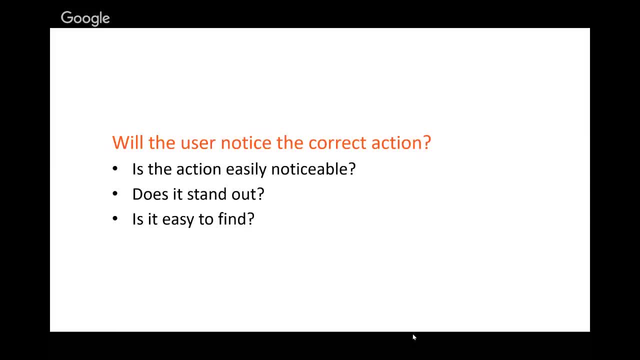 You know, do you have a reason to go to that far right-hand side? Probably not. The other thing I recently tested with one of those buttons on the right-hand side was when it zoomed in, it actually laid over the text, so it overlaid some of the text. 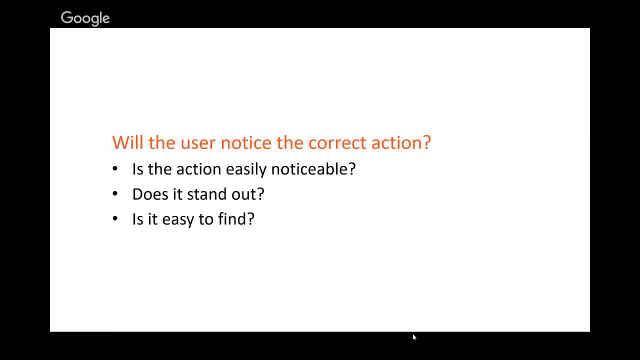 as you did, browsers that were zooming, So that actually obscured things as well. Another instance that we find often- and it's nice to see it being picked up in WCAG 2.1 earlier this year- was: can you actually see where you're meant to enter some of those details in a form? 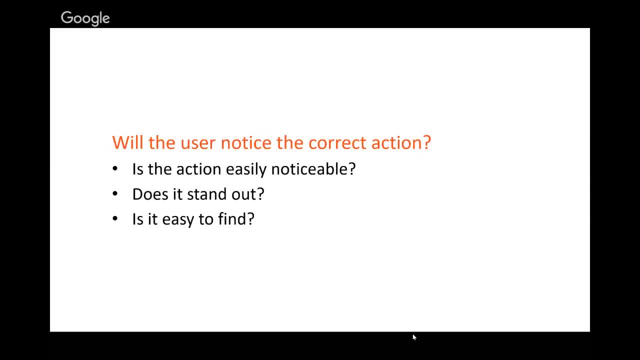 A lot of forms have very, very pale outlines and it's hard to differentiate the text entry box from the background. And then we've got other design patterns that have been coming in where they were applying underline, instead of a bounding box, an outline box around those text entry fields. 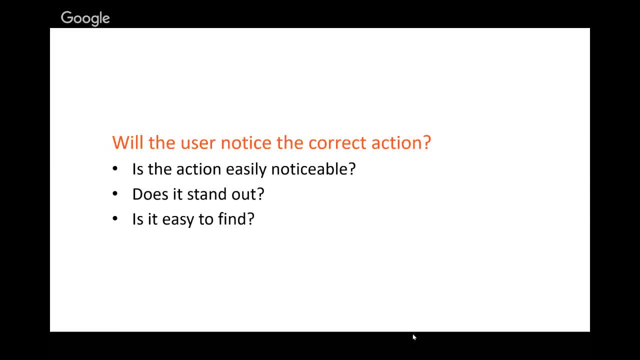 And you know people think: OK, what is this? You know there's nowhere for me. they want me to. they were trying to collect some information from me but there's nowhere for me to type it. So you know it's not just. is it easy to notice? 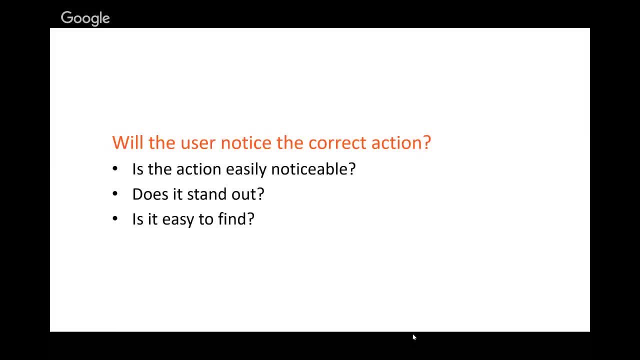 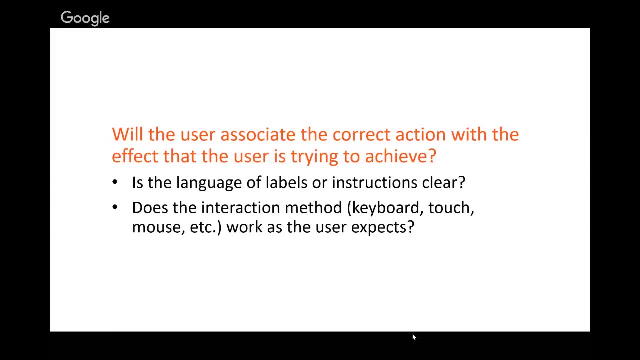 but as we said in the first thing, previous slide about the questions, is it something that they're expecting? Is it meeting their expectations as well? So the next question is: will the user associate the correct action with the effect that the user is trying to achieve? 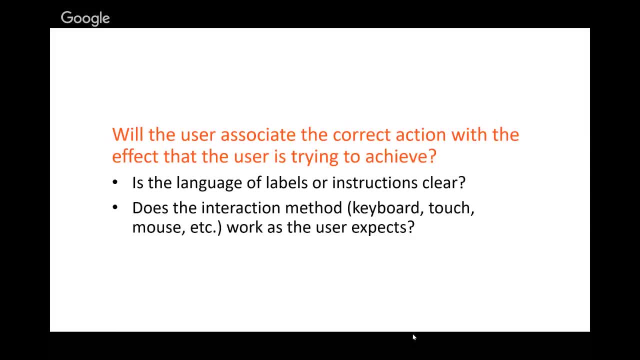 So this is where you know, first of all, language. Are labels or instructions clear to users? And of course this can take many forms. It can be. is the label clear? Is it visible? I keep saying I've got an allergic reaction to placeholder texts. 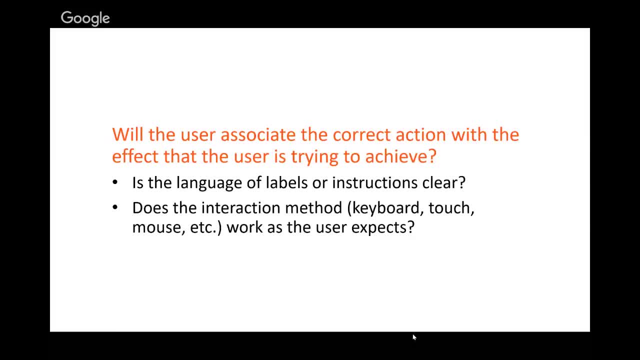 because when you tab to it it disappears. So you know, all of those type of things sort of play into this particular question. And does the interaction method work as the user expects? Link underlying text tends to is expected to take the user to another part of the screen. 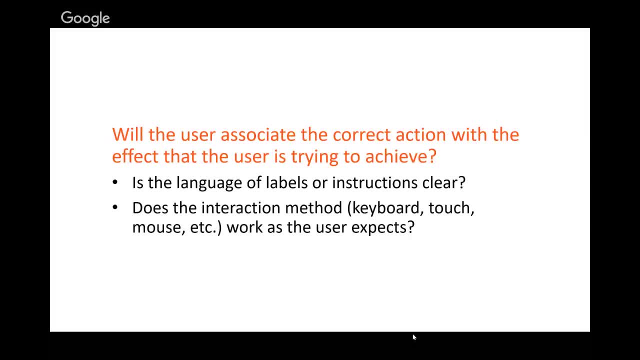 or a new screen. Something that looks like a button is meant to actually perform something, typically on the page. So you know, we've built these expectations up by over a decade and a half now, And if you make things behave differently, you're making the user actually work harder. 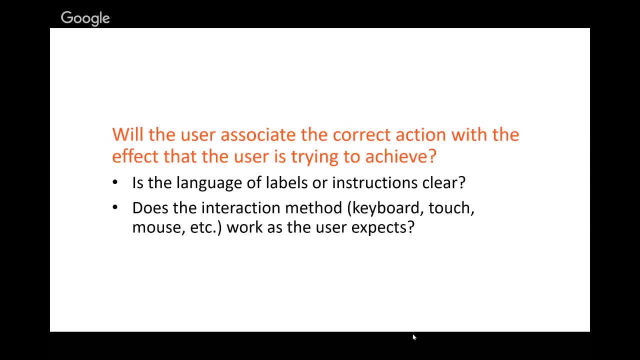 to understand what's going on Now. additionally, you've got a button there, but it's been coded to be only available to a mouse user, And the person with their touchscreen keeps touching it and touching it, and touching it and nothing happens. 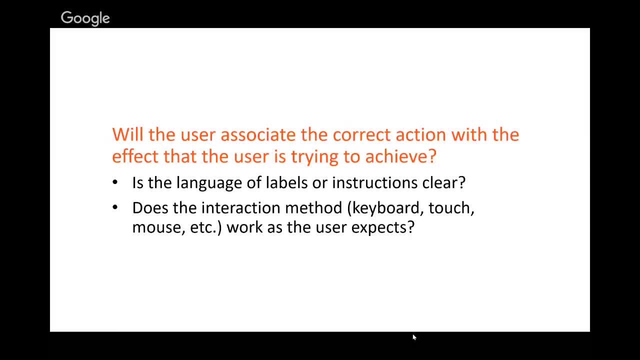 So you know, the interaction that they're expecting is just not available to them because of the way things have been built. So these are the types of actions that we're looking for as we walk through in Joe's shoes or Jill's shoes. 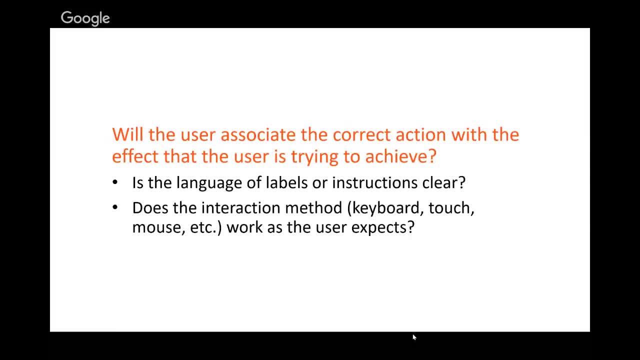 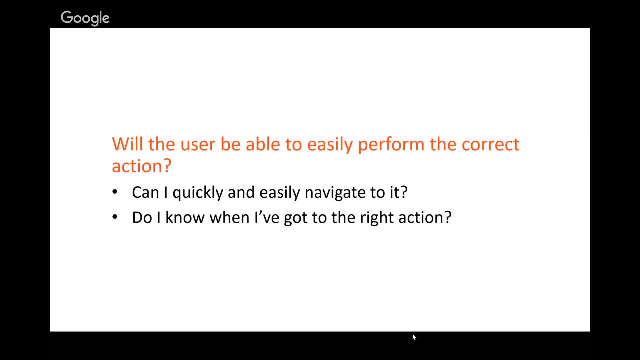 or anybody else's shoes, And are we getting those types of? can we understand what's expected of us and is the interaction what we expect? And that dovetails really nicely to the next question which, as I mentioned, was one we specifically added. 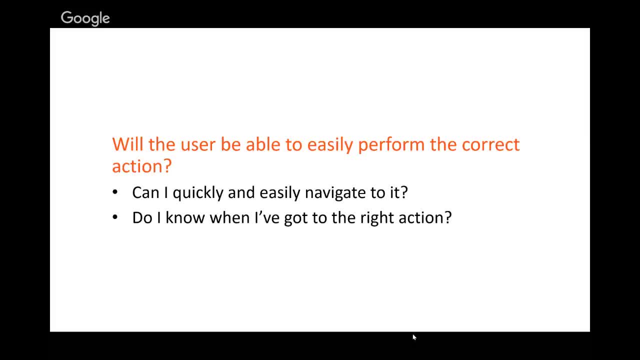 to this sort of set. that's often used. So the next question is: how can I quickly and easily navigate to where that action is? So this is not just being able to use the particular button component text field. whatever it is that we're looking at. 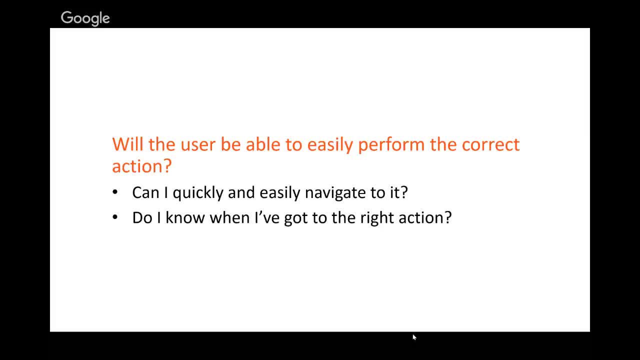 but can I quickly and easily navigate to it? So that's picking up on, really you know. to go back to our calls, example: do I have to tap 90-odd times, you know, to get there or not? Can we easily navigate to it? 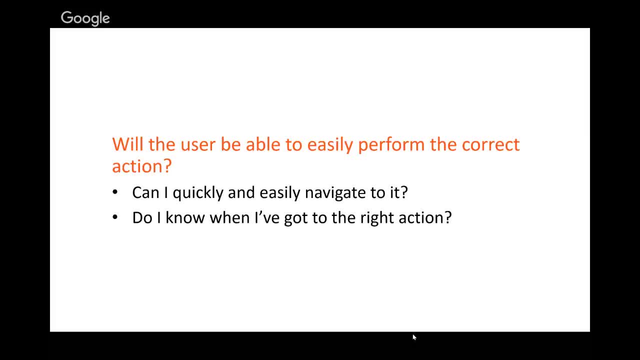 So that's picking up on, really, you know, to get there or not, Can we cut down to 60,, 30,, 20? You know things like that. And it's coming back to that general principle of you know, putting the most important information first. 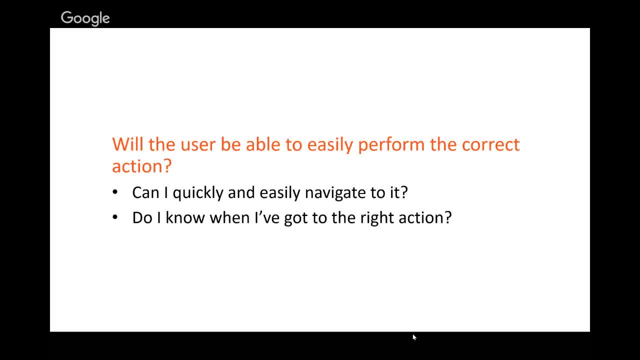 or, in this case, putting the most important interactions first as well. And do we know when we've got there? And this really brings back the for keyboard users in particular, that focused indication: how many screens have we all tabbed through? if we've tried tabbing through? 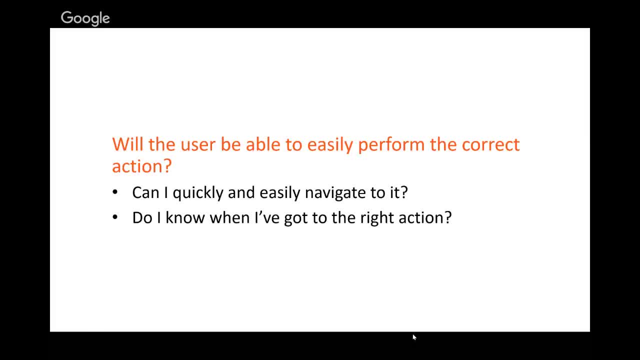 and you just lose track of where you are completely So how do you know when you've got to the right action in order to be able to undertake that action, to complete your task? It's really, really critical, And I know many of us have long arguments. 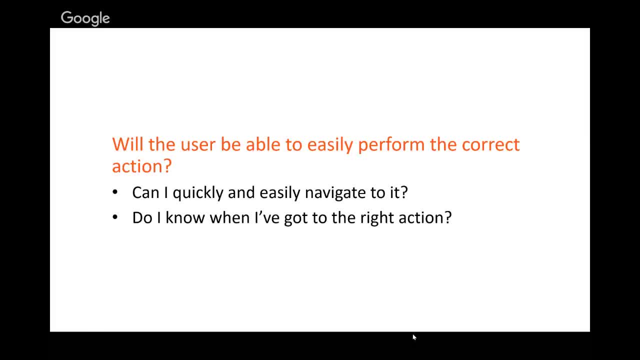 with graphic designers in particular because they want it to look pretty. But the argument that I often use with them is: it's for the keyboard-only user And if you've got to show that to the product manager, the senior executive, they're not going to tab through the page. 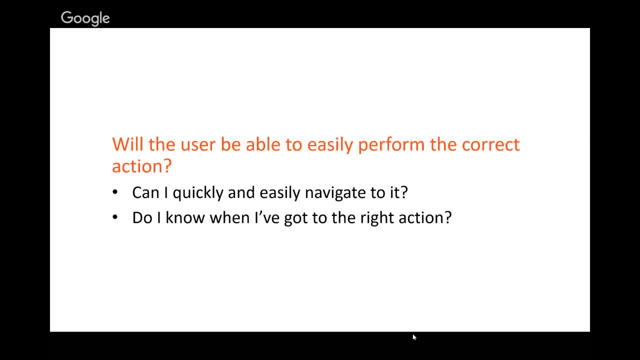 They're not going to see what you've done behind the scenes to make things easier for people who can't use a mouse. They're going to use a mouse and a keyboard. Highly likely that they're going to use a mouse and a keyboard. 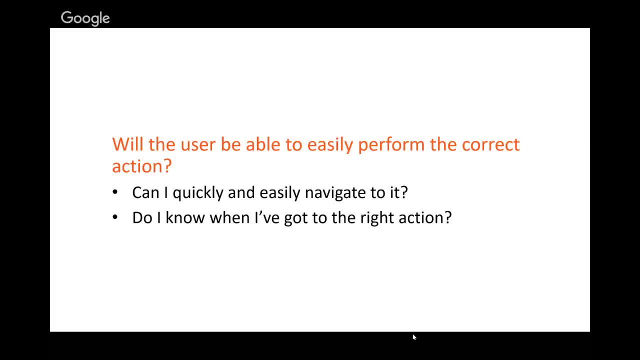 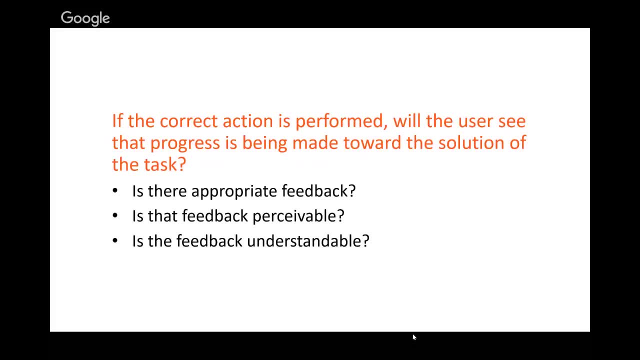 If they don't use a mouse and a keyboard and rely on the keyboard to navigate, then they're going to appreciate what you've done for this group of users. And the last question, I guess, brings us to our goal, which is our task. 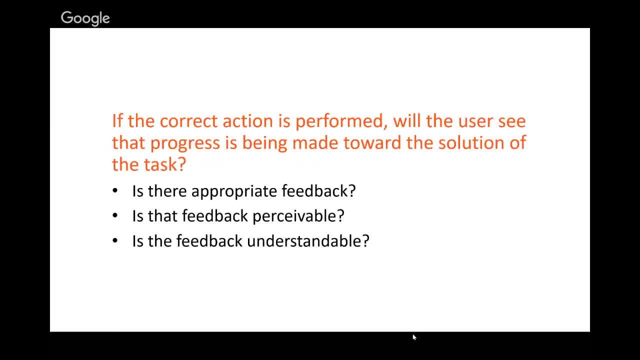 If the correct action is performed, will the user see that progress is being made towards the solution of the task. So is there appropriate feedback? Do you know that you have done something correctly? How many times have we seen a form where you submit it? 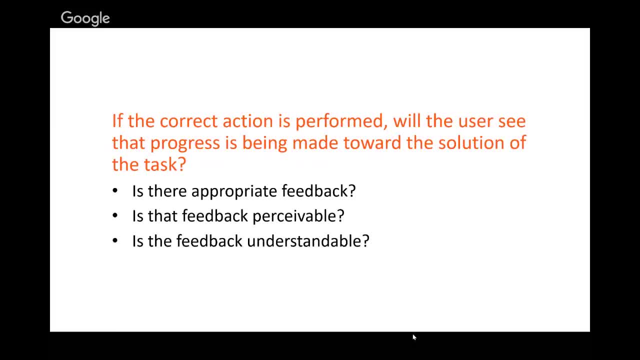 and you get no feedback. It just, you know, goes to a new page or even just reloads a blank form Or leaves you with the data that you've entered there, Even though you've pressed submit. And from the, you know keyboard user or screen reader users. 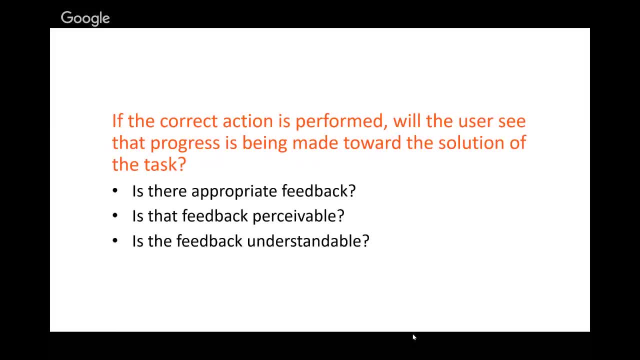 the focus stays on the submit button, So they press it again because they don't know that anything's actually happened. There is no feedback necessarily provided to us visually, or to somebody who's listening to it or to somebody who might be tabbing through it. 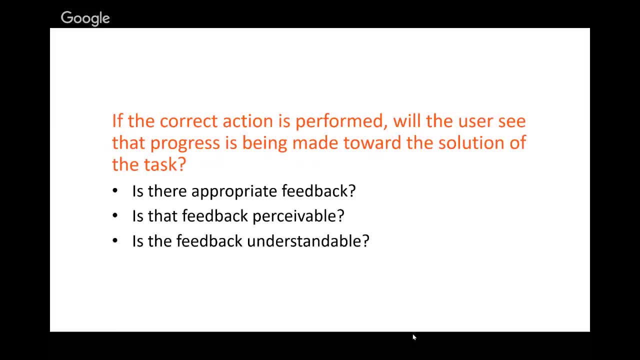 and the focus still stays there on the submit button, And that dovetails into the questions of: is it perceivable? Can we see it To build on that example? Andrew, screen magnifier users as well. If you submit a form, you've got the success message actually up the top. 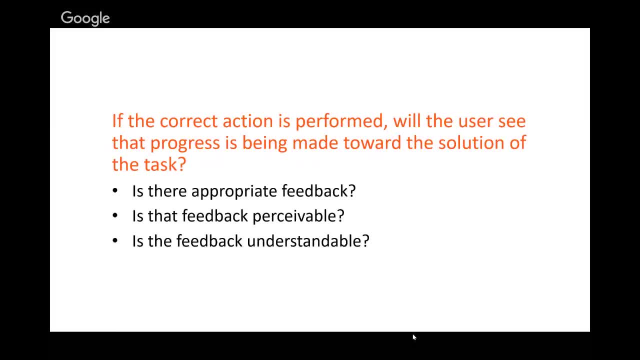 and I did review a site where I sort of pinged them for this and funnily enough again it's not a WCAG compliance error- Like I can't actually fail it against any particular WCAG success criteria, But if the focus stays, you know, down the bottom on the button. 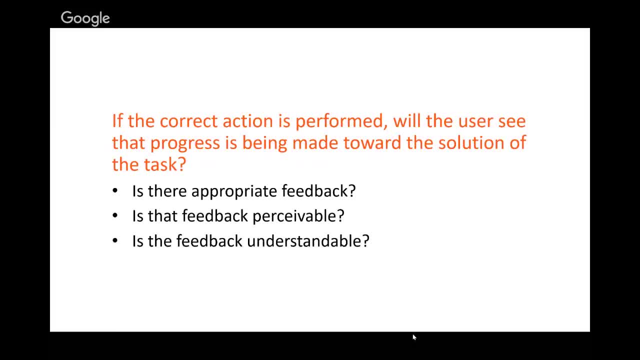 and the success message at the top. that's forcing that screen magnifier user to go searching for success or failure. So again, really great feedback. Actually I keep that whole screen magnifier thing. I reckon the best thing is: old school, get a piece of paper. 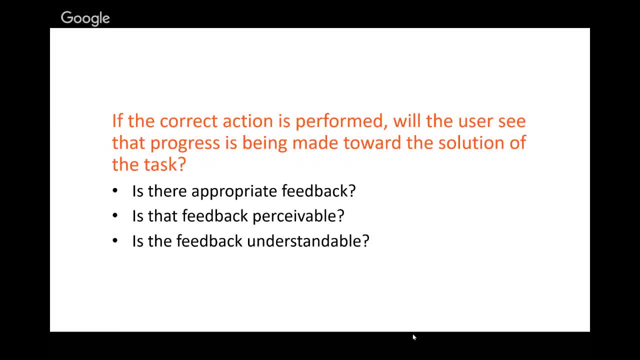 cut a window out, stick it on top of your design and then do your cognitive walkthrough through that small window and just manually move left, right, up down to simulate that sort of you know magnification. Yes, you can do it with tech. 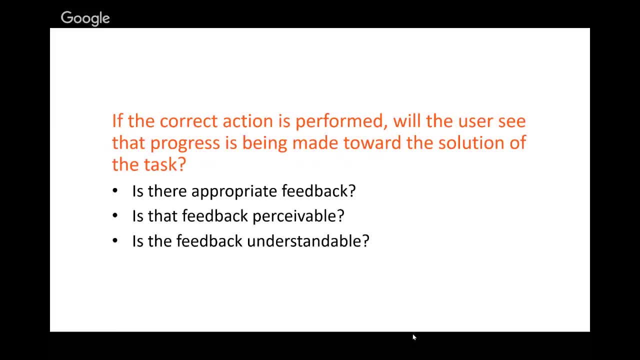 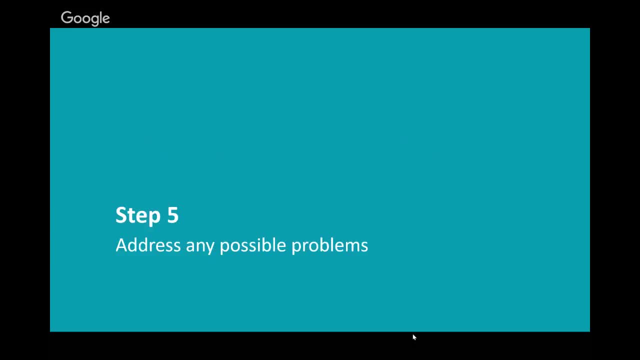 You can fire up magnifier on Windows or Mac or what have you, But I think it's nice to do a bit of a paper-based exercise. Lo-fi exercise- Yes, Great. So we've identified a couple of problems and, as I said earlier, 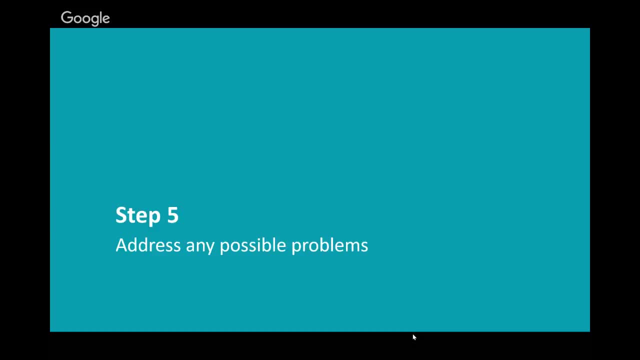 if these are significant problems. there's no point in getting Jill or Joe- our two personas from earlier on- in if they're not actually going to be able to complete this task anyway. So we need to be able to address these problems before we bring real users in. 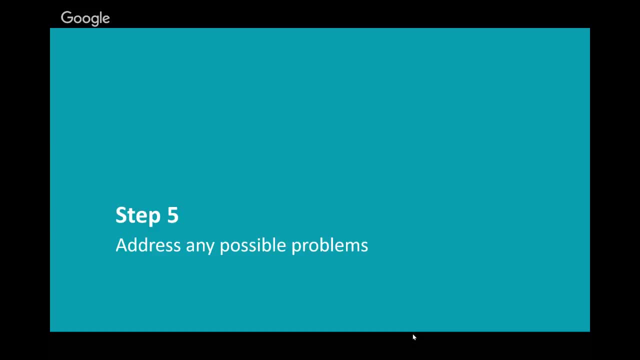 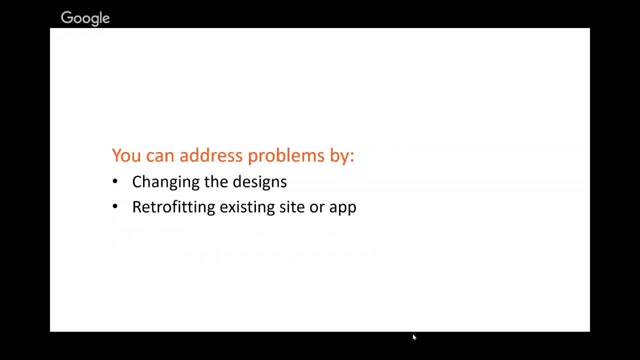 So this is part of our debugging: effectively to make sure that things are working before we start testing with people who might be relying on these assistive technologies in the way that we don't. So, really, there's two options. You, of course, identify problems, change the designs. 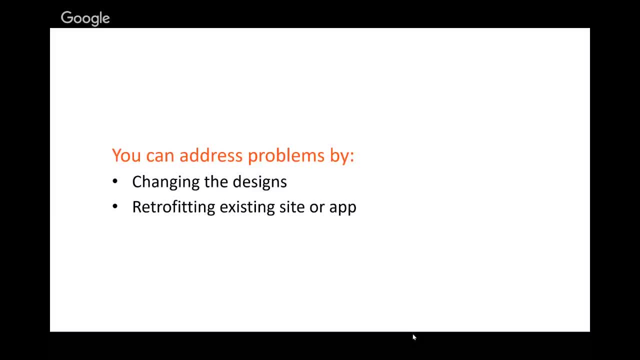 or if you're using this process on an existing website or app, then you're probably looking at retrofitting or fixing those issues within the existing build. Yes, as Coles did, to put an additional skip at the top of the screen to skip to the login and to skip to the shopping cart. 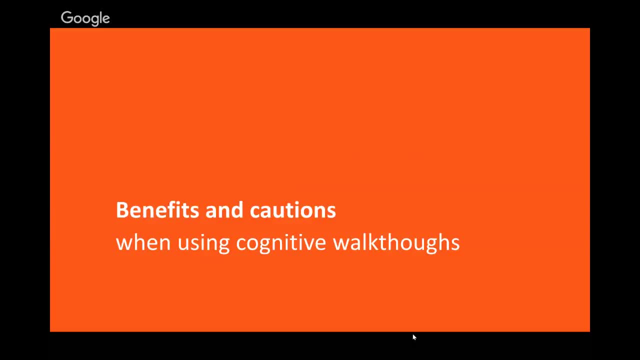 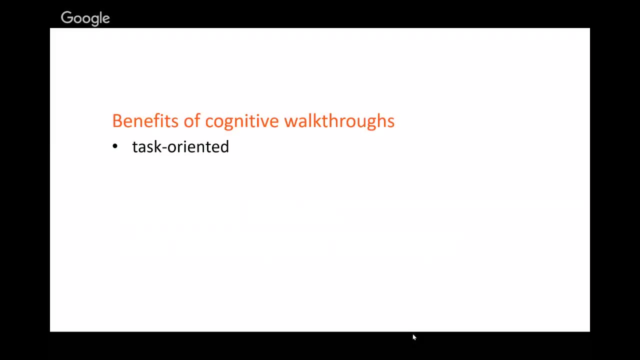 So there's a whole lot of benefits, but there are some cautions when we're using this approach. The benefits are that they are task-oriented, which, when we're doing accessibility analysis typically, or accessibility reviews, we do tend to look at the components. 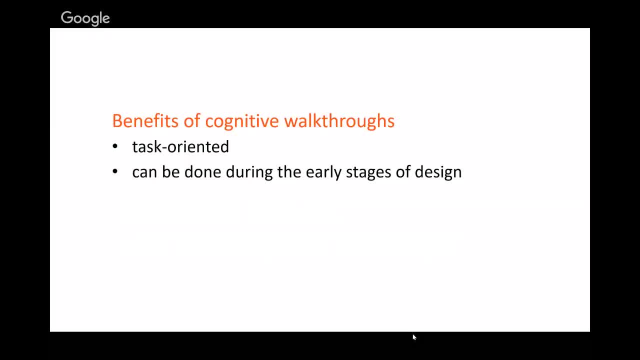 rather than the overarching process. What the customer is expected to do from end to end is often overlooked. They can be done at an early stage, as Sarah was saying, even with paper mock-ups, If we cut out on another piece of paper a little window and we move. 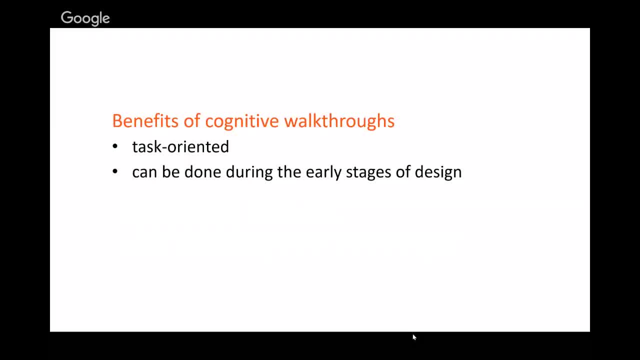 that around on the screen to simulate what a screen magnifier user might have to do to get through the 16 screens, to go from well login to checkout. That's probably the perfect one to go visit a colleague you know and say, hey, here's some paper printouts, let me give you a task. 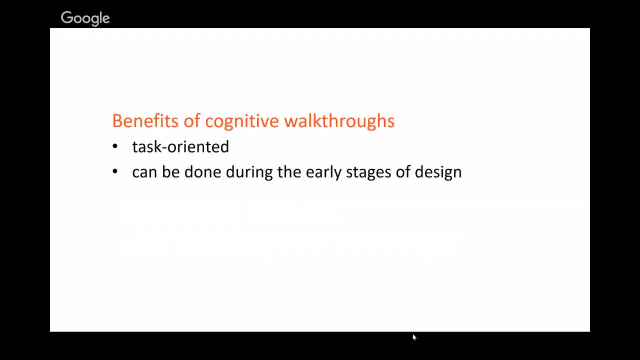 but actually I need you to complete this task within the window Yes And see how they go. We can identify requirements, gaps here, things that might not have been specified in the original specification for building this product, even if it's going through an application. 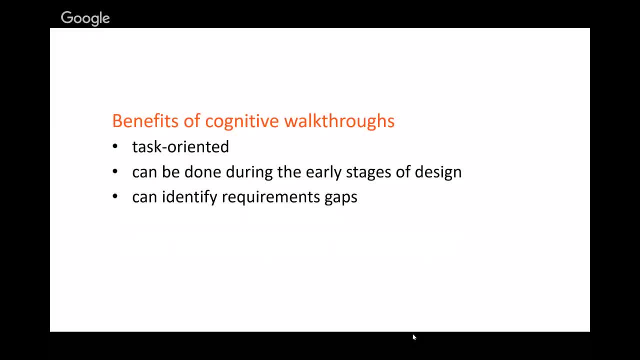 Even if it's going through an agile process, we tend to still have some overarching requirements that we may have missed entirely. Obviously, it's faster and more effective than true usability testing but, as I say, it's not a substitute for it, but it means that we can get a lot. 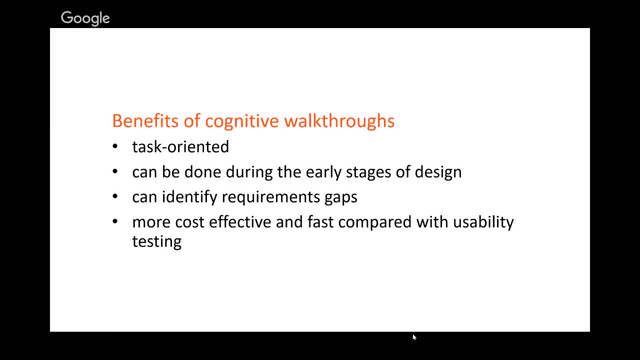 of issues out of the way early on by standing in Jill's or Joe's shoes- one of our persona's shoes- and going through the process as though we were them And trying to complete an entire task rather than looking at the individual components on a page and do they meet the WCAG success criteria? 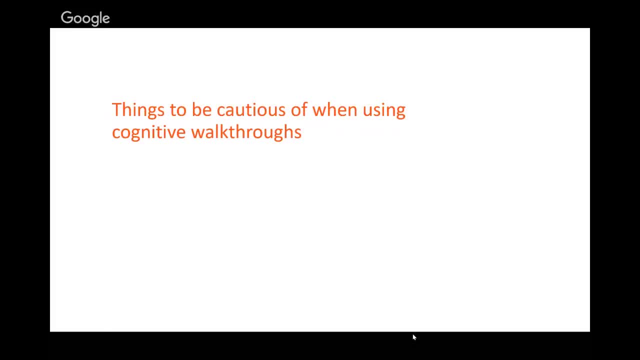 So there are a few cautions around cognitive walkthroughs, and we've kind of foreshadowed the first one, which is that it's not a substitute for usability testing, which we will keep saying Certainly, yes, this is not a replacement for putting something in front. 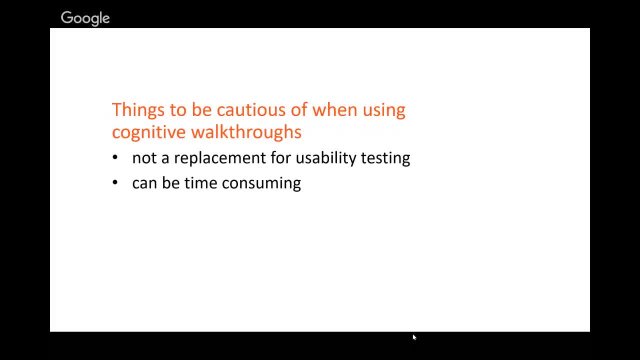 of real users that are using different assistive technologies, adaptive strategies, and bring everything else they have to the table. Yes, So you know there's definitely that Cognitive walkthroughs they can be time consuming. So when you think about, let's say, our example of eight web for everyone, 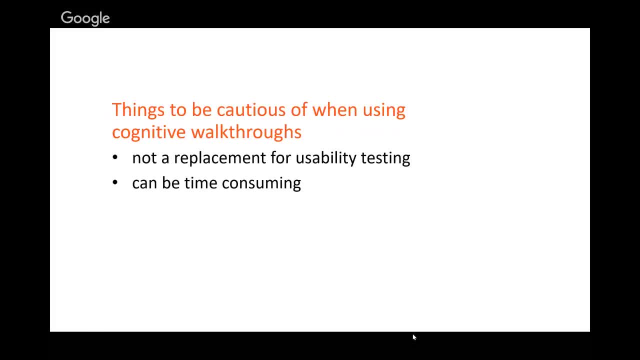 you know personas times by. I think it was about six e-commerce tasks. you know that's getting pretty easy, That's getting pretty high up, So it can be a time consuming process And probably you get your best insights when more than one person actually does. 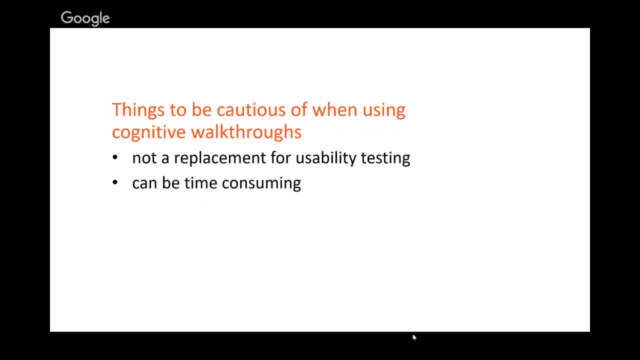 this process with a persona and a task. So for me it's about balance. I've had people you know sort of ask: oh so how do you choose which personas to do? And for me, you know, there's no hard and fast rules, but I probably use the ones. 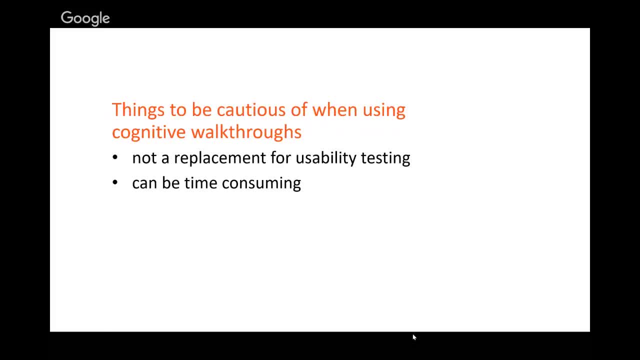 that might have you know that I might be less confident about Or haven't sat down and really considered the experience of that particular user, So it's a little bit of a judgment call. I think Yes, And you know we don't need to. I mean even with usability testing. 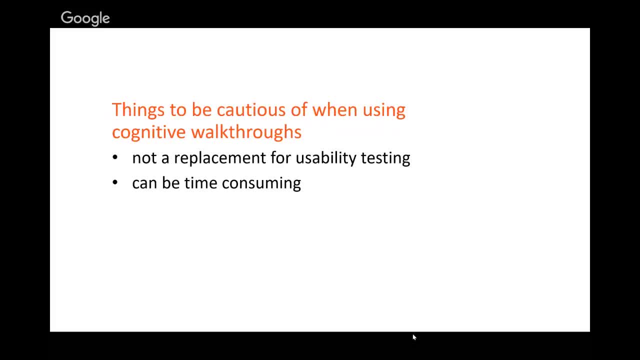 we're not testing every different ability, every different way that people might interact. You'll probably find, if you do a couple of the tasks with a couple of personas, you're going to find some common problems across those. You say, okay, we've got to fix these across all the tasks that we're expecting. 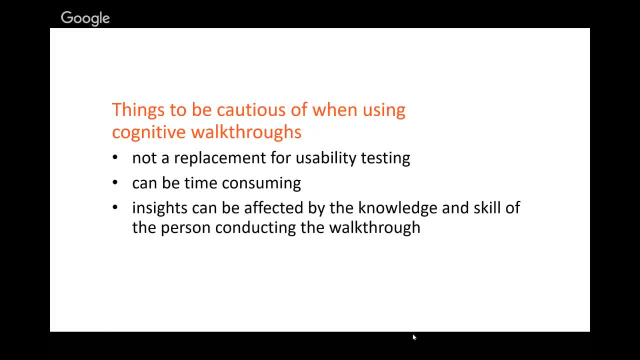 We've got to figure out what we're expecting people to undertake And, lastly, the insights can be affected by the knowledge and skill of the person conducting the walkthrough. So I sort of alluded to this when we chatted about the personas and how the principles could help alleviate a little bit of that. 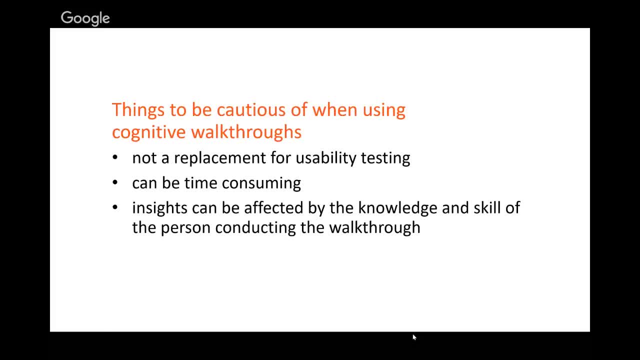 But you know, for Andrew and I who, well, Andrew's been in this game longer than I have. but you know we've got a fair bit of insight through the time we've spent, you know, in accessibility With users. 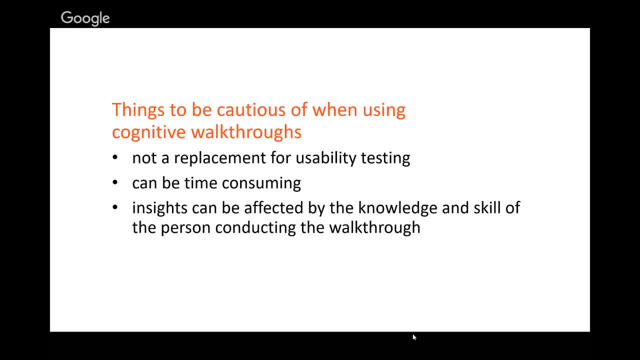 And so you know, I guess, for us we draw on that knowledge. So there's always a little bit of a risk that the knowledge and skill of the person conducting the walkthrough can skew the results a little bit. And also, if you're too close to your product, let's say you know. 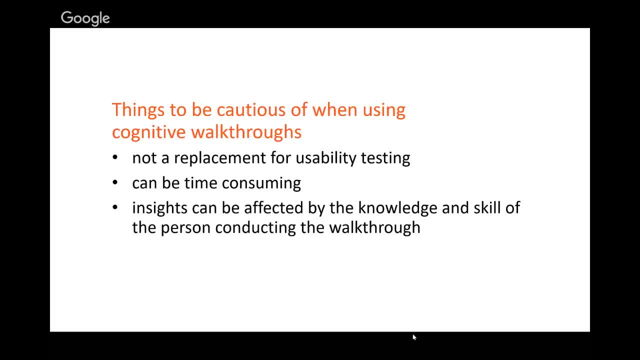 you are the designer and you're the one doing the cognitive walkthrough, then sometimes you know you can make wild assumptions or just be so used to the interface that that might also You know what to expect. Yeah, that's right. So that's why it's always nice to you know. 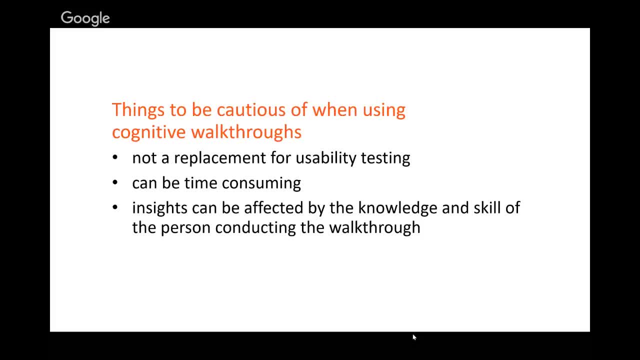 Get a colleague, or Exactly. It's kind of like a bit like the guerrilla testing, where you know you run around to your colleagues and they're the first stop you know for your guerrilla testing to say, hey, you know, what do you think? 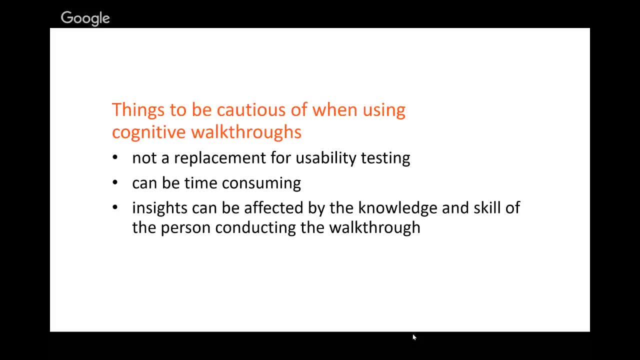 you should do here And I think you know, for cognitive walkthroughs. this is the same. It would be great to get people involved And it's a good team activity. to be honest, It's the start of you know, talking about the experience for the user. 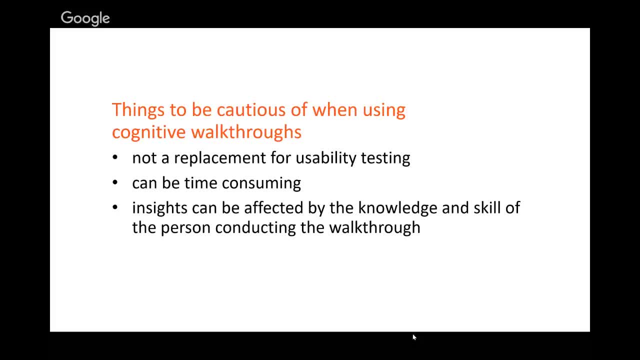 So get your developers as perhaps one of your people you might be doing the walkthrough with, or your testers, or that kind of thing. That could be a really great way of also getting the team talking more about accessibility- if they haven't, And raising some of that. 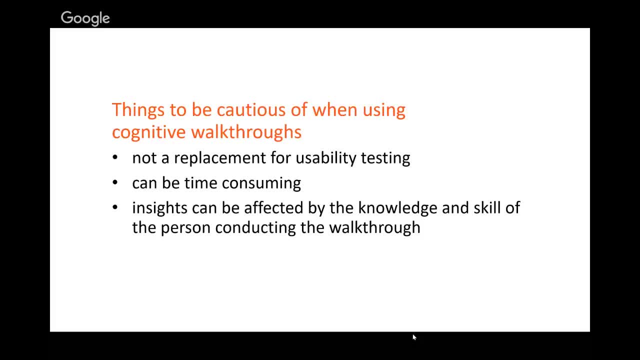 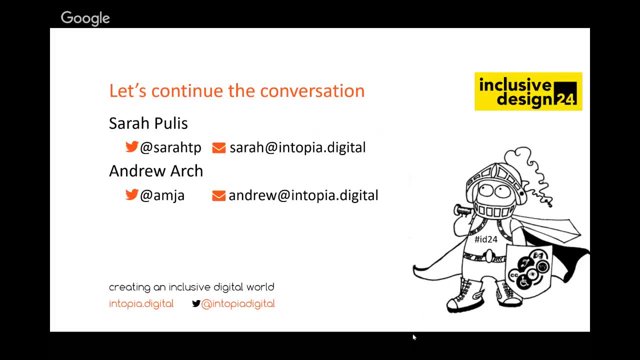 Starting to raise some of that empathy with the way that different people might have to interact from the way that most of your development team are probably going to be interacting. Yeah, Okay, So that's about all we wanted to say on that topic. The slides and everything will be available on the ID24 website later on. 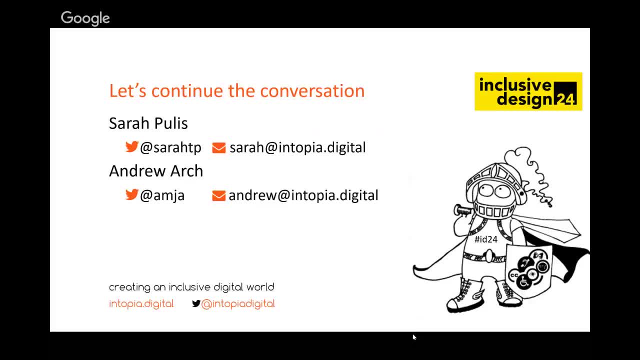 But we'll also post those on our own website. Any questions, Ian or Rinaldi? Hi, That was a really great talk. I think that's just going to be a really useful tool for people. I think it's going to be a really useful tool for people. 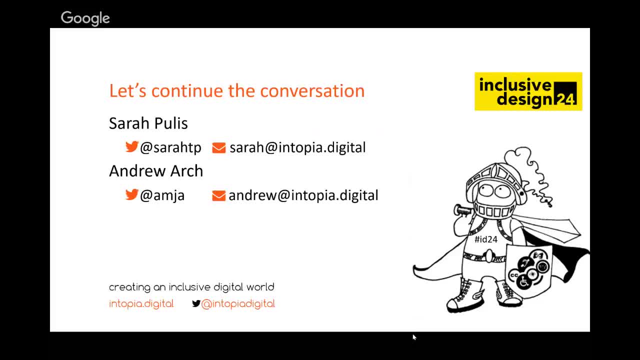 I don't see any questions on Twitter that have come through, but I have some questions myself, actually. So do you find that this is something that designers and developers really embrace, or is this something you have to persuade people to do? Do they see the value automatically, or is there a way to sell this into teams? 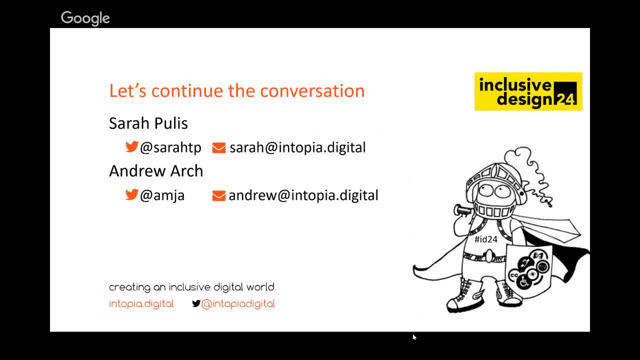 The clients that I'm working with- I think Sarah will say the same- are keen on accessibility. That's why they've engaged us. They see this as a quick and easy method of doing some quick checks to be able to walk through some of their designs and then some of their builds, some of their MVPs, quickly. 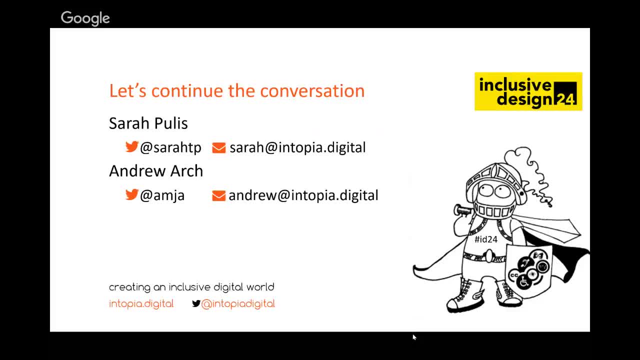 to say: have we made some big mistakes? So some of them are embracing it quite quickly, Quite openly and quickly, no persuasion needed. They just see it as another tool in their overall usability toolbox in many respects, because we're often working with the usability and the UX people to make sure that things. 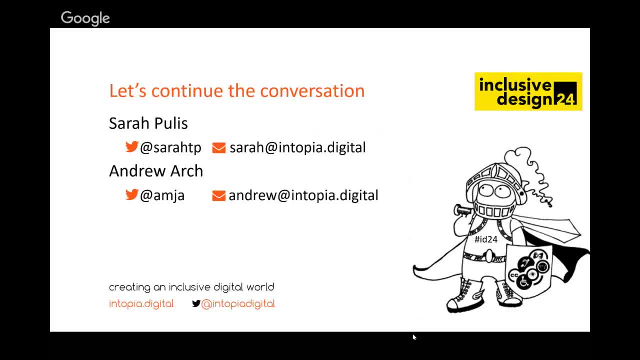 work for the broadest range of people. So what we do have to do is then persuade them that they still need to get people who rely on assistive technologies or adaptive strategies to come in and do that final test. Some of them are quite open to that. 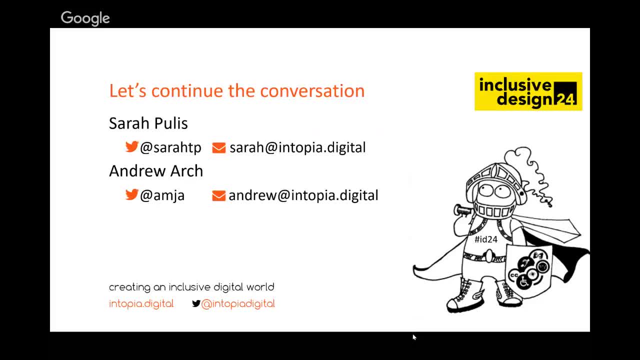 Others say we don't have the budget. Will this do So? no, we tend not to have any problems with getting them to adopt this approach. They may not adopt it to the extent that we might like them to. with all eight personas and 16 tasks. 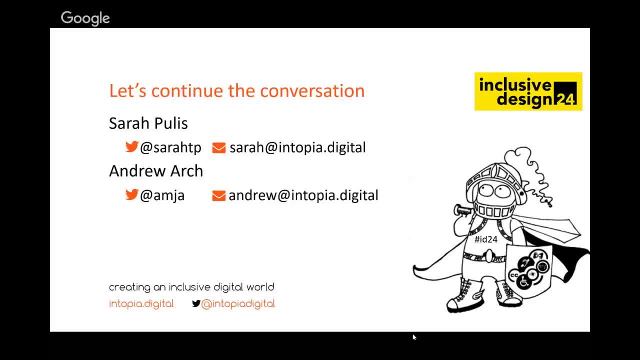 They're quite open to trying it on their products, just to some extent. But, as I say, the next barrier is then persuading them. Look, you knew what to expect, So you knew how to step through this the way, and all you've done is made sure that there. 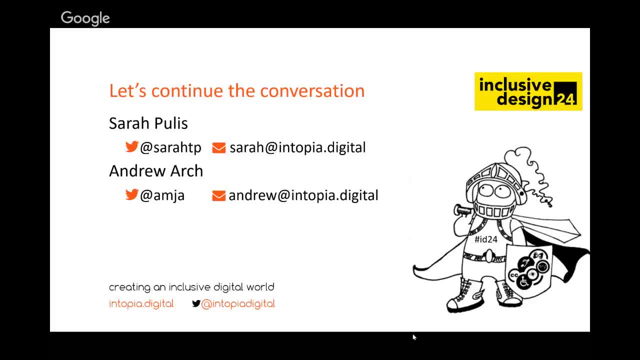 aren't any serious technical barriers or serious potential usability barriers, like the 90 clicks to get to the shopping cart. You still need to check with people who are relying on this, Don't understand your website, are coming to here. You want them as a customer. 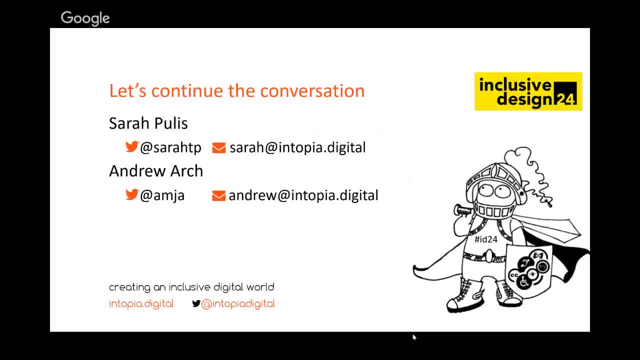 Bring them in and do some real checks with long mouse users, with screen readers, With screen magnifier users, with a dragon voice dictation user and different people like that, because then you're going to find out a whole lot more on what you'll find out. 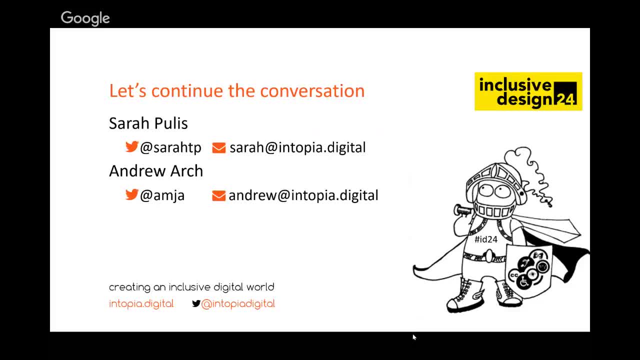 Then we'll probably highlight some what you might perceive to be or other user usability people that you come in for usability testing to be a minor usability issue. But people with disabilities will have to highlight these as a much more serious usability issue And if you can fix it for them, 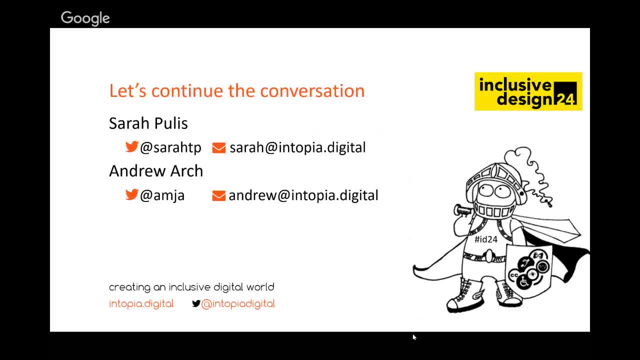 If you can fix it for everybody. I've also found it's actually a great teaching method as well, So I've integrated this into our designing for accessibility and inclusion workshop, And it's a great way of you know again putting someone in the shoes of the user. 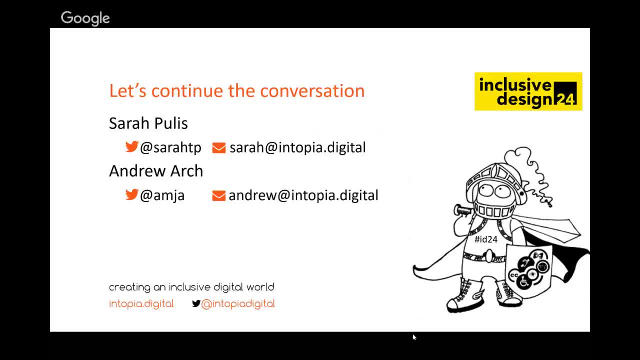 And usually I do that on something that's already existing on their site- and get them to do that cognitive walkthrough process with one or two personas. Come back, do it in sort of small groups, Come back together, Share their insights, And that both cements what we're sort of talking to them about, about how to better design. 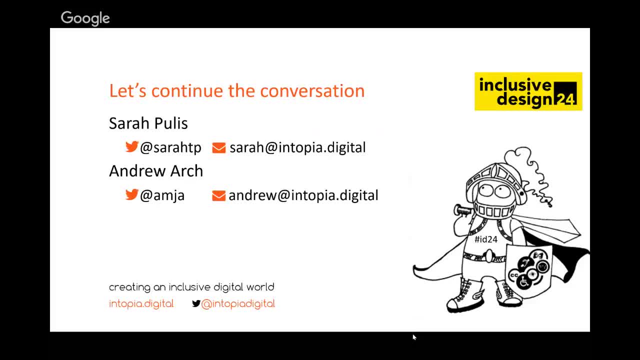 for diversity. But I also feel that once they've done that process, particularly on one of their own websites, where often then you go back and then you, because it's a live website, and you say, oh, and by the way, you know that assumption you made, that it works this way. 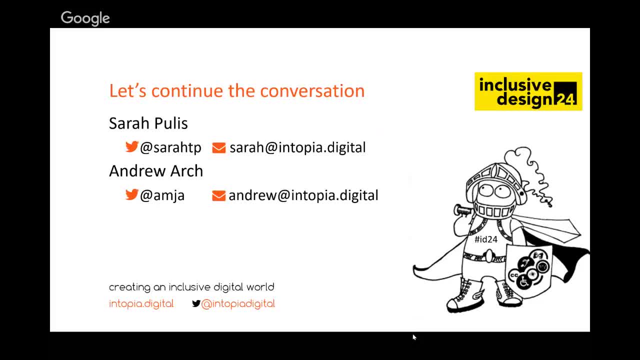 or what have you actually it doesn't. It's only like, oh, I see the value of this And you know, realize, yeah, It can be that light bulb moment. Yeah, That's right. Yeah, You talked about it being, you know, potentially time-consuming, but it's. I'm sort of equating. 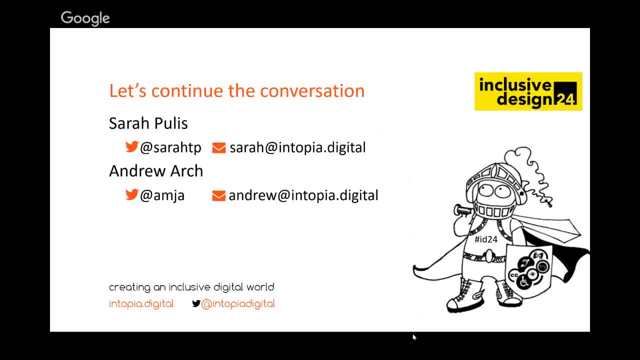 it with. something I've always told developers, in particular when it came to doing usability testing, is that you wanted to make sure that you already found things like missing alt text or links with no accessible name, The things that you can, you can find, you know, basically with automated tools before. 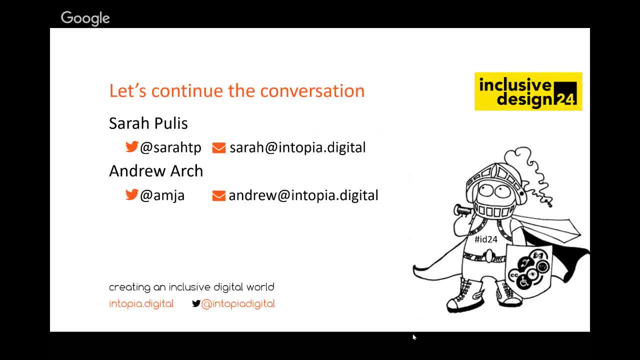 you go to usability testing because it's cheaper to find them beforehand than to find it when you're doing testing with real users. So you can kind of save on that, you know. so being a bit more prepared and having done some of the work yourself, I think would really help. 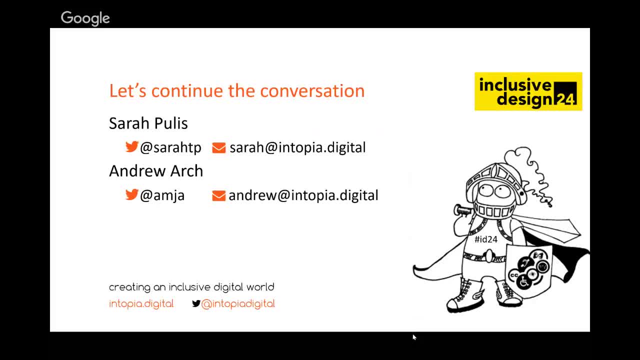 Absolutely Sorry. Go ahead. Sorry, I was just going to say So. there are certain users that you can do more than the pen paper or prototype testing with. sometimes you know certain low vision users if they're using just screen magnification. 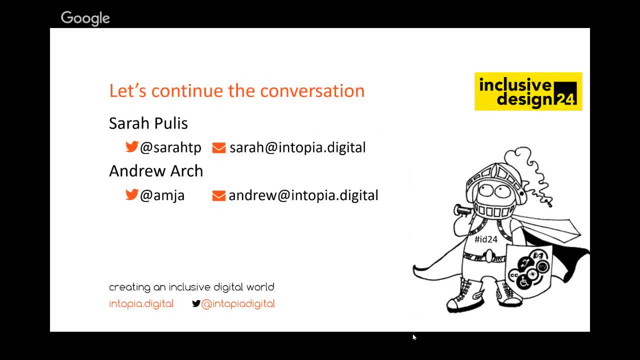 you can still do it on a sort of a click-based prototype, but you can't do that for your assistive technology users like screen readers and dragon and what have you- until you actually have a semantically- you know- meaningful development. So for me it's also invaluable. 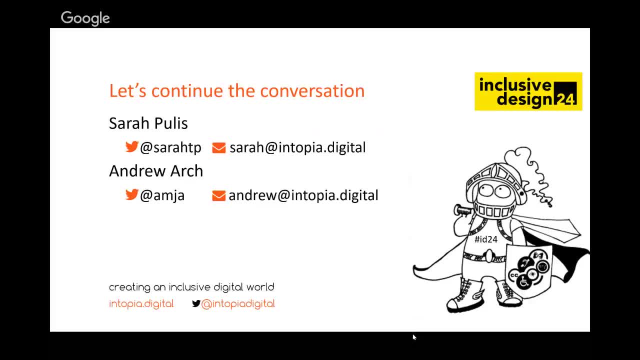 For those sort of types of personas where we can't really test until later on in a traditional way. So again, it's, you know, walking through before we get to that development point, And of course that that saves time If you walk through, find some issues, update your designs or recommend accessibility requirements. 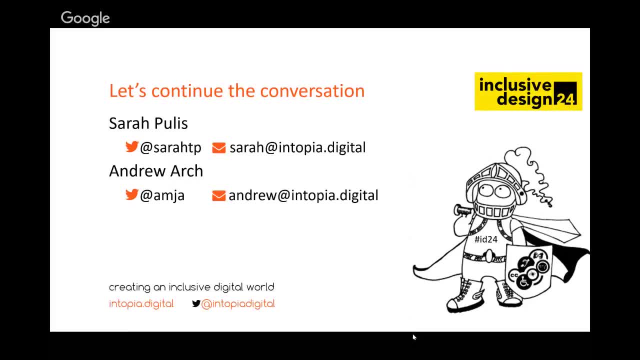 based on that, Hopefully you've got less issues at the end. you know whether it's from a compliance point of view or coming out of usability testing as well. Great Rinaldi, do you have any any questions? I was also going to ask about the challenges and like persuading people as well to actually 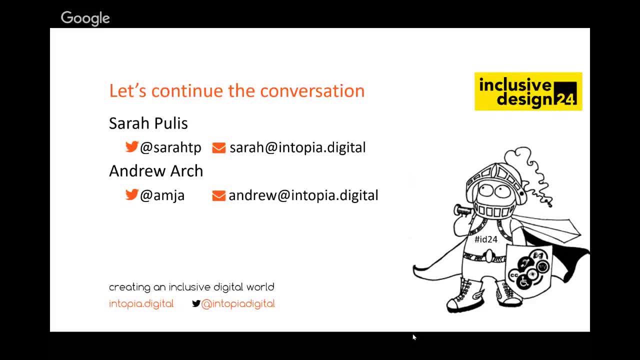 adopt the this kind of cognitive welfare approach to usability, because I think it's a very insightful presentation as well. But yeah, since it's already answered, I think it's that's more or less for it for me, but maybe you'd like to also mention some resources you'd like to recommend for people to get. 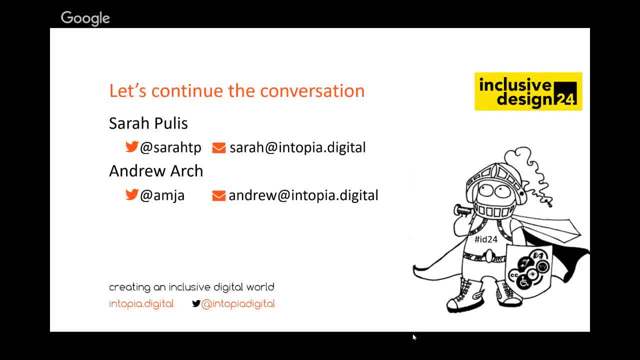 used to cognitive walkthrough as well for people to perhaps like get used to adapt. adopting the approach Resources: I'm not sure there's a lot of resources out there around not cognitive walkthrough specifically for inclusion. Definitely the personas that we mentioned from a web for everyone: govuk and Barclay. 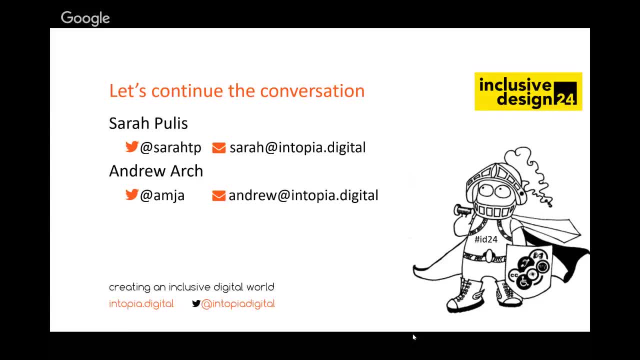 and Barclay's help with that persona side of things. Probably the tasks will be already done as part of the UX, but I actually don't think there's a lot out there. No, That's why we've chosen this as a title for the talk, because we're not. you know, it's. 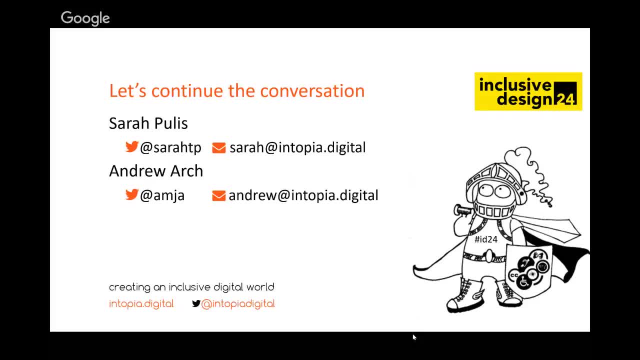 something that we've adopted, but it's not something that we've found much literature about how to do it from a range of ability or disability perspective compared with. you know, the traditional. you know walking through. okay, can I click here? 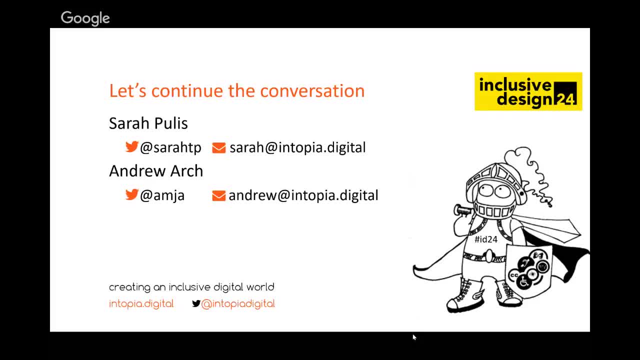 Can I click there? UX perspective? Well, the good news is, this video will be available on YouTube after ID24 is finished, And so this is now one of the resources that we can point people to Great. So I have one more thing to ask you about is one thing that I've been doing- is you. 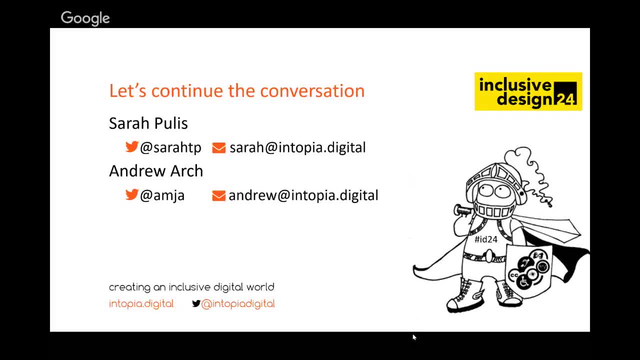 know, suggesting to developers that when they're doing, let's say, sprint demonstrations or, you know, whatever demonstration they're doing of their work when they've completed it, that every so often they do this just using a keyboard, for example, just to get. 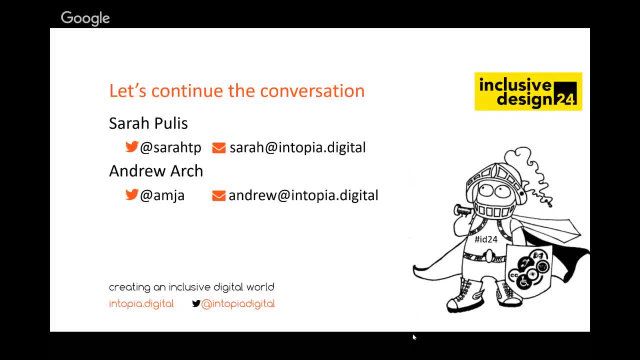 into the habit of thinking about using a keyboard to use whatever they're building and to get other people on the team used to seeing things being used with the keyboard, And it feels like this could be. you know, an approach to take is not just demonstrating. 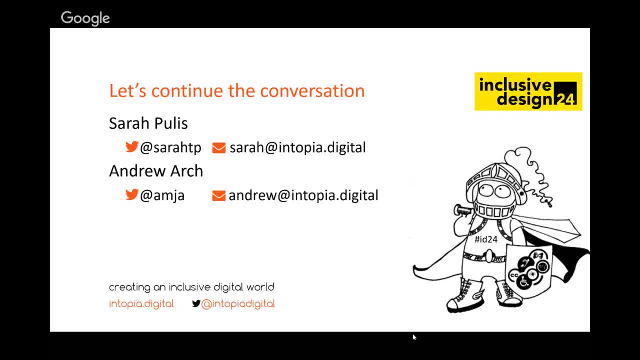 something with a keyboard, but demonstrate your work as one of your personas. Do you think that would work? I like that idea of bringing that into the sprints on a regular basis. That's very nice. Yeah, I have seen some teams actually do demos like what you said at. yeah, sort of sprint demos. 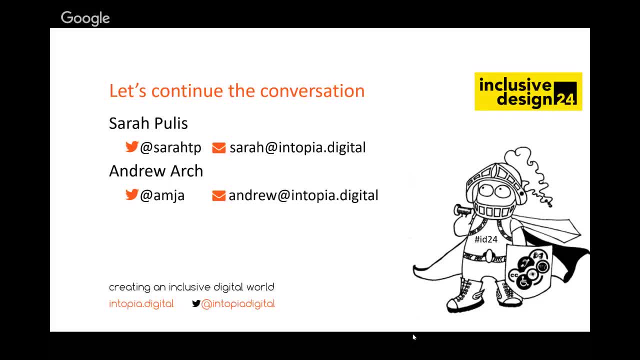 to show the accessibility. But I think the power of bringing that to the table, The power of bringing the persona into it is, you know, essentially attaching it to a user, So not just, hey, I can tap around here and look, it works great, you know. to actually.